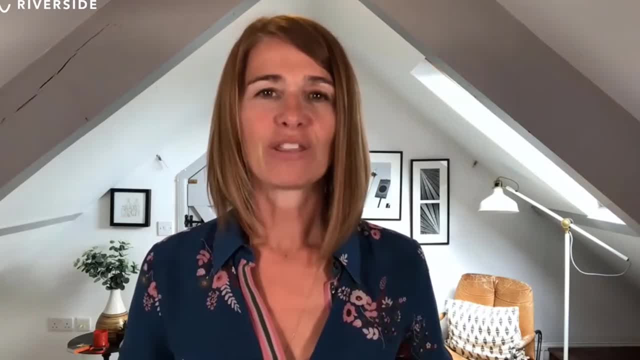 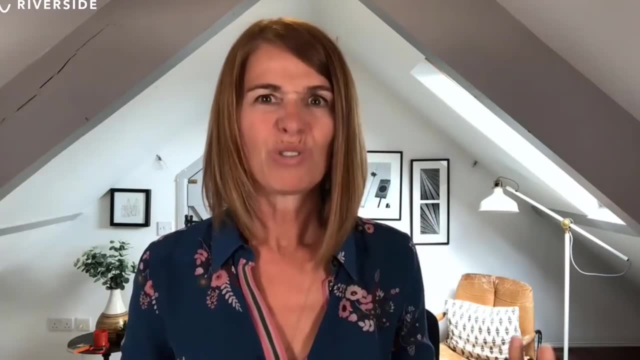 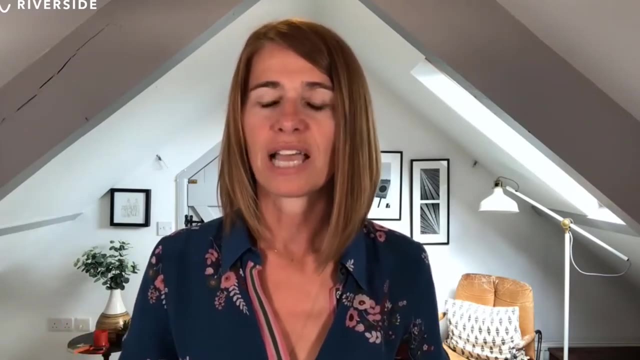 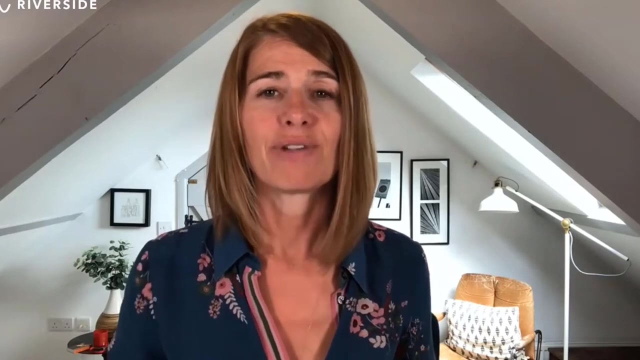 your argument? Is it evidenced? And then ethos. Ethos is really about credibility, And he looked at it in two ways: Lived in credibility. So do you say and do the things you promised that you would do in order to understand the content, And do the things you promised that you would. 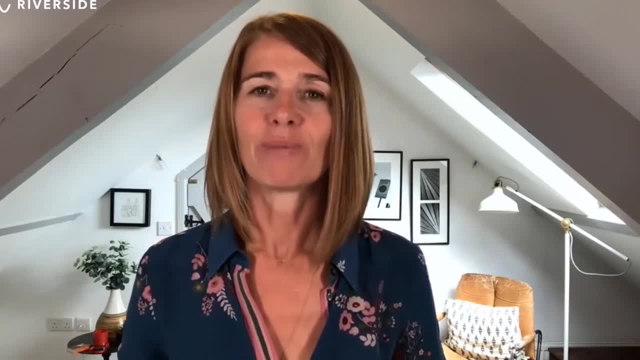 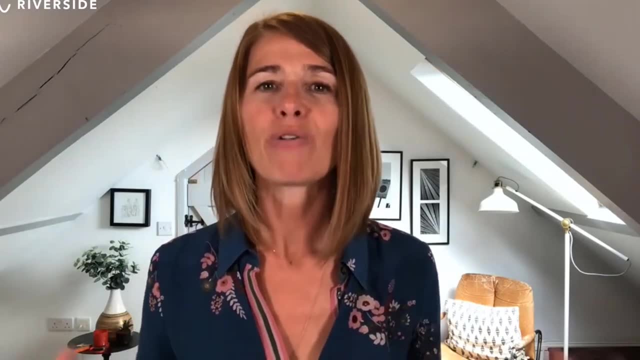 do in order to understand the content. Did you look at it in two ways? Did you look at it in two ways? Did you open up your emotions? Did you look at it in three ways? Were you going to look at it in three ways? And then let's say that every good speech you do has 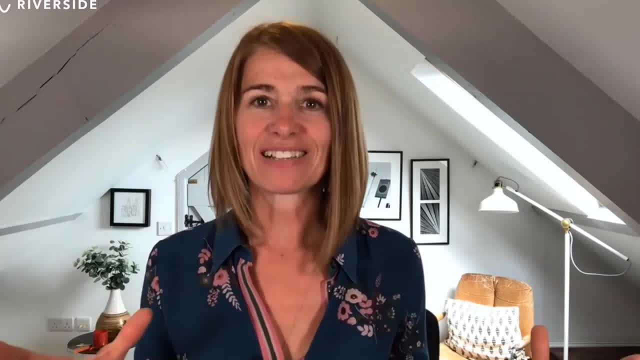 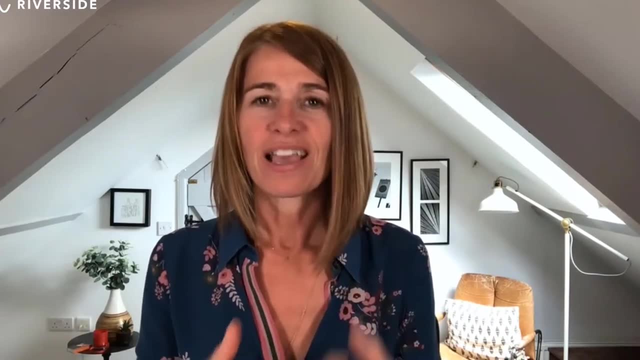 these two things right: The purpose, the purpose of speech and the purpose of Seventeen. today we are going to be discussing speaker credibility. How do you create that credibility with an audience almost instantaneously, so that they are buying into you and buying into your? 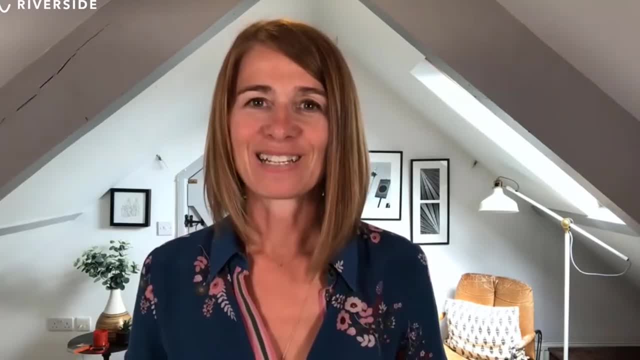 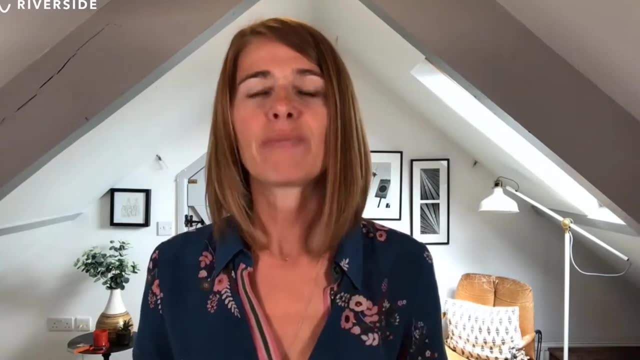 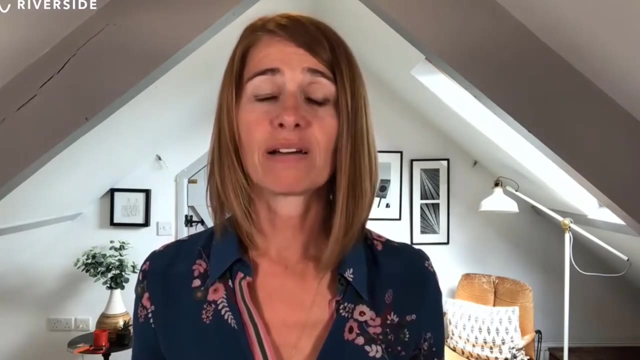 content and listening from the beginning to the end. So, before we get into the kind of what of all of this and how to do it, I want to think about why. Why is this important? Well, as a woman who works with females in leadership, in entrepreneurship, 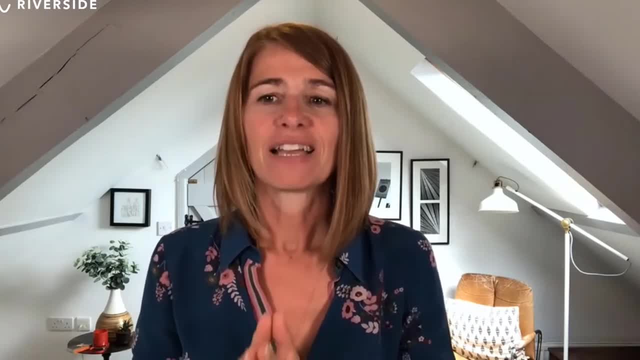 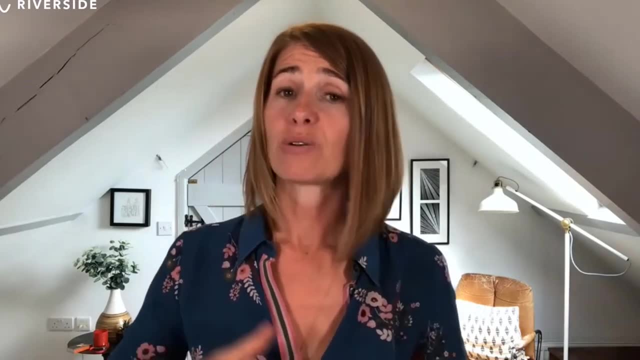 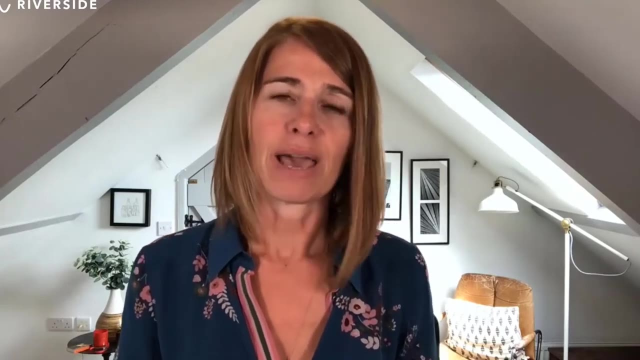 women are still getting very little investment in terms of entrepreneurship. Now, what's interesting is that women, whether we're in the corporate space or in a startup space, an entrepreneurial space, we work harder and longer than our male counterparts. We perfect our work, We spend. 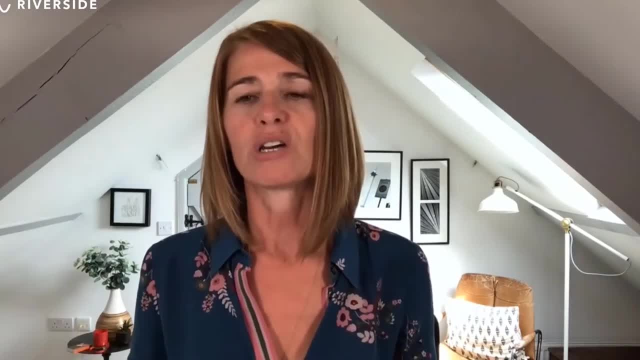 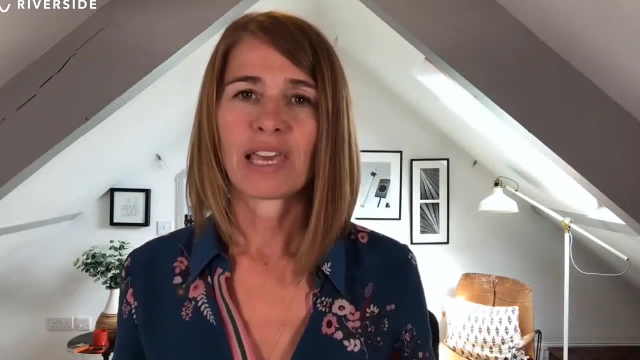 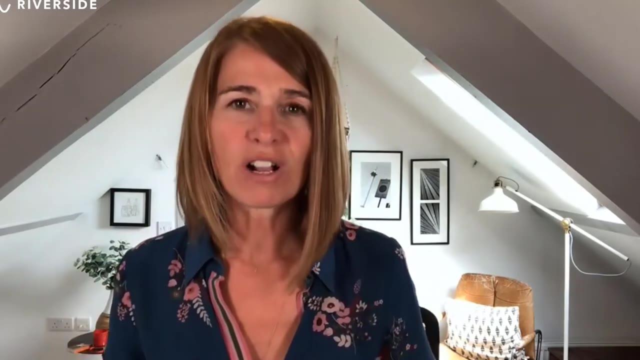 a long time Getting things really, really good. But those are wasted hours if we don't ever spend time thinking about not just what we're going to say, but how we're going to say it, And not just what we're going to say, but how we're going to structure what it is what we're going. 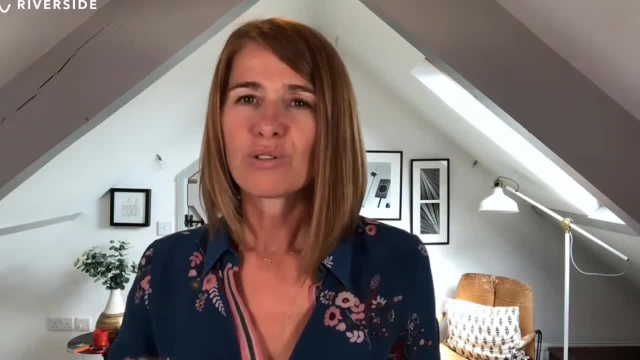 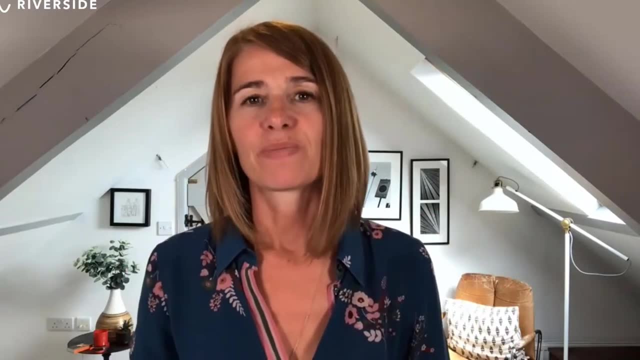 to say, and how is that relevant to our audience? So it's not just what we say, it's the order in which we say it and how we say it that is going to make a difference. So I really want us to start with that. 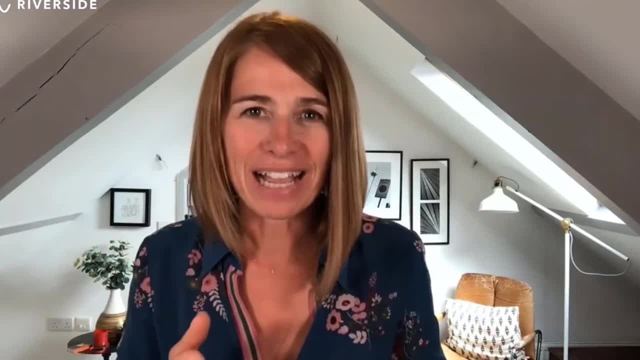 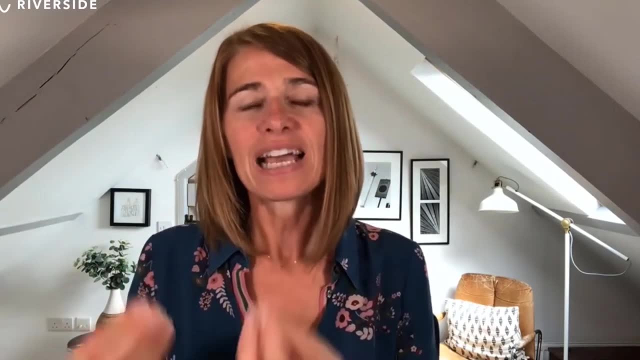 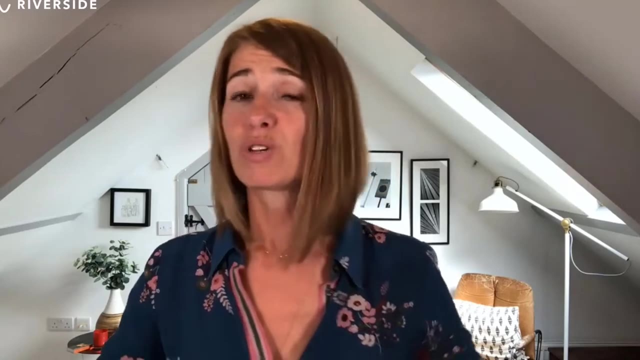 I want us to stop wasting time and gain back time so that we can do the fun stuff, the living bit of life, and not just perfecting our work, and so that we get impact when we actually do that. And I've spoken about this before and if you've watched any of my other videos, you 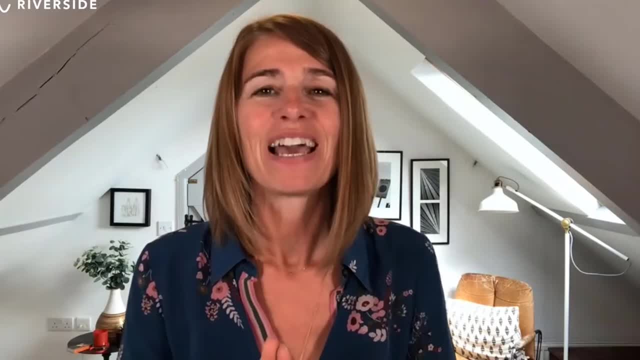 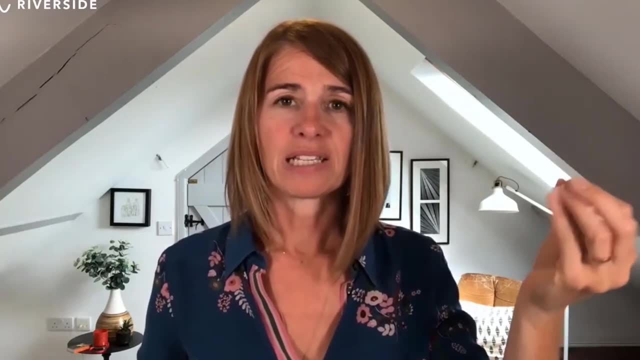 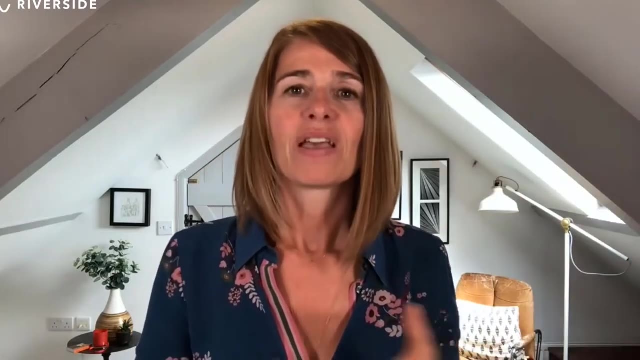 will have heard this many times over and I will keep saying it till the gals come home: There is a relationship between how we are perceived in terms of our competence and our and how we deliver. So a poor idea- sorry, a poor delivery is equated to a poor idea. 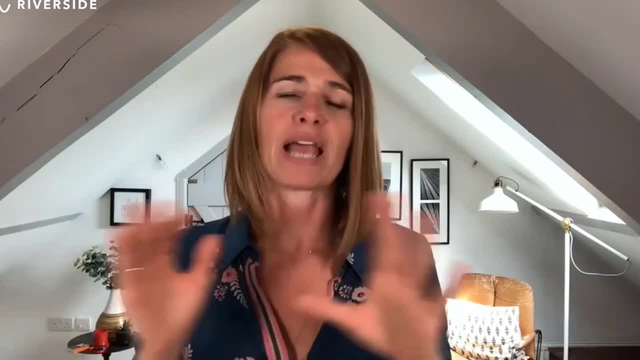 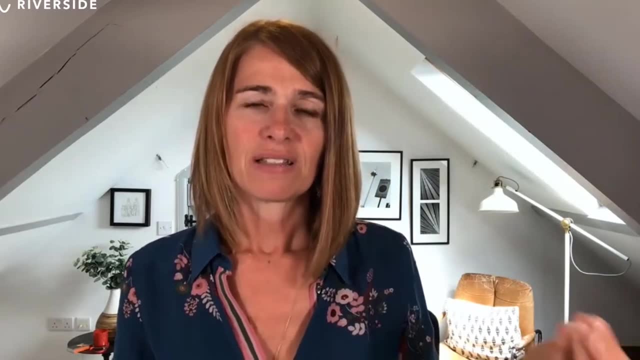 You could have the most brilliant idea. You could have perfected your deck. You could have spent hours, days, months, years perfecting your idea, But if it isn't credibly delivered, then that idea becomes a poor idea. Equally, you can have a brilliant idea And if it's brilliantly. 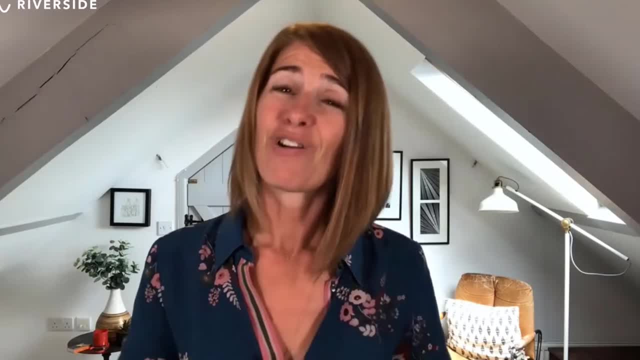 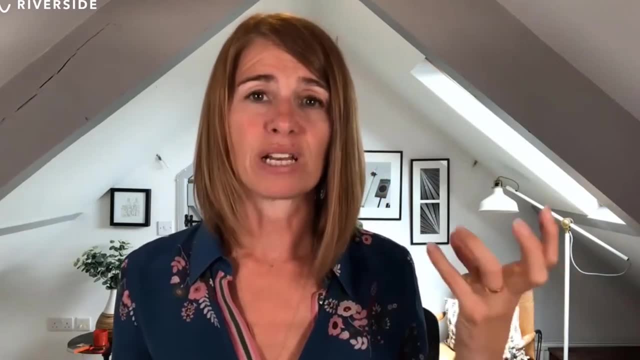 delivered. the two things become equated And there are occasions, sadly, where if something is brilliantly presented, but it's a terrible idea, but it gets taken up because it's brilliantly presented. So what we want to do is find that sweet spot where we have fantastic ideas that 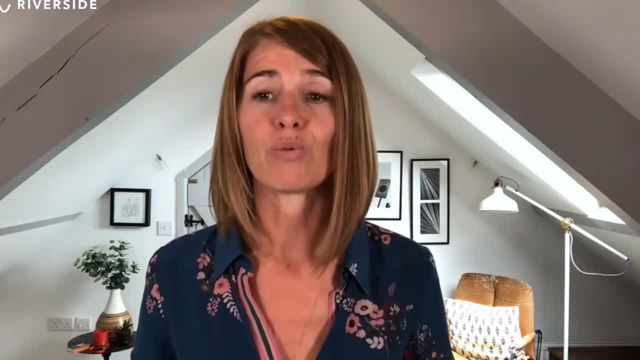 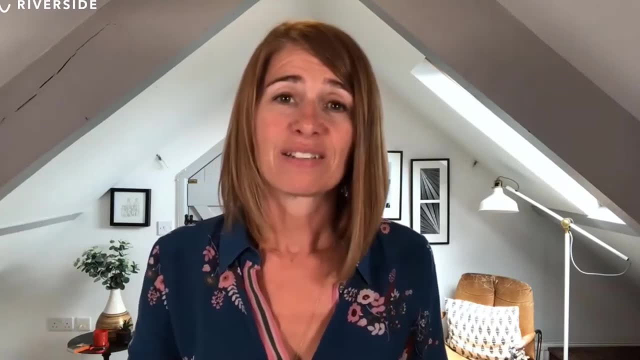 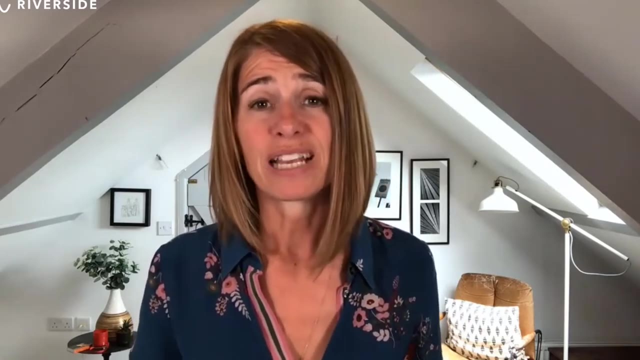 are brilliantly presented in a really, really credible way. Now, if you are in the entrepreneurial world, why is this important? Well, as I said, women are still only getting about 3% of all Investment, So they're not getting the venture capital that they need. because the presentations 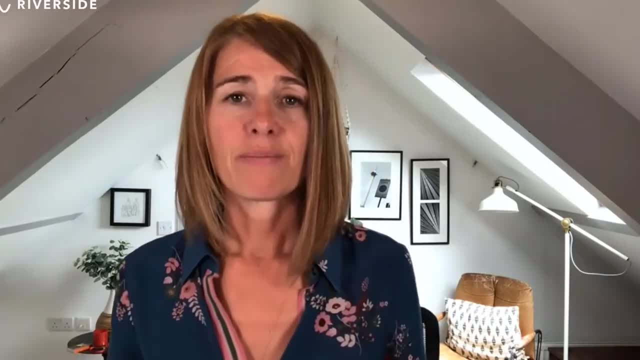 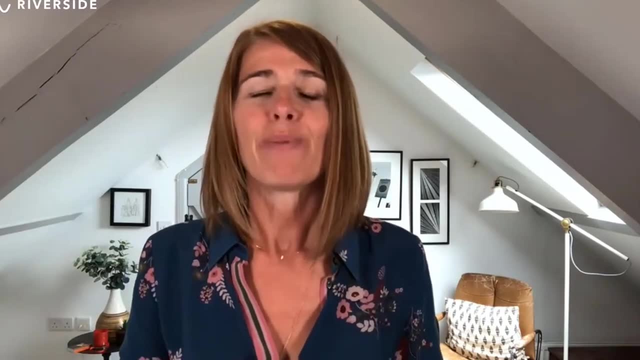 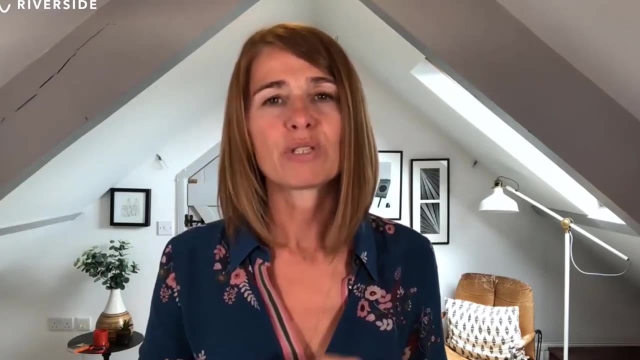 their pitches are not as credibly delivered as men. Now there's also there's a lot of other biases going on there and we haven't got time to dive into all of that today, but we could certainly make that better. It means that every time you do a sales call, every time you're. 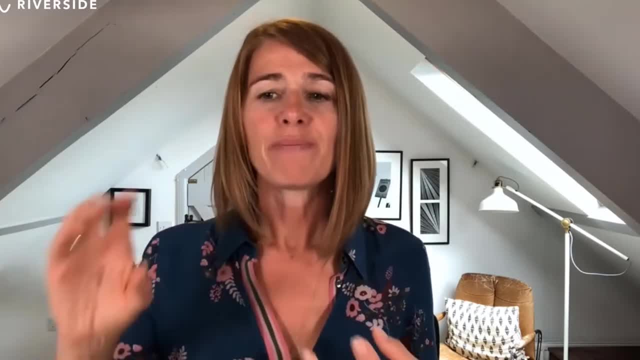 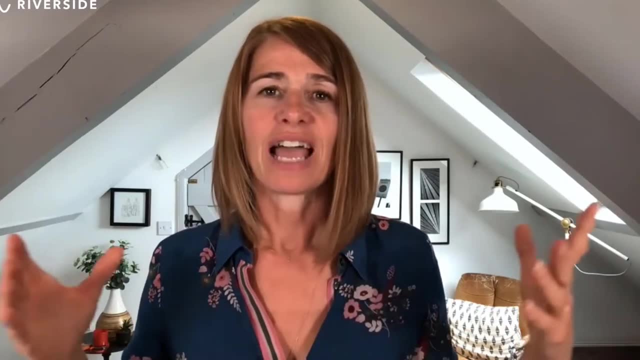 speaking or negotiating with a client or a supplier. it means that every time, you're doing everything you can to make sure that you're getting the best out of your business. you're ernealing anything on social media, So lives, recordings like this, Any videos that you 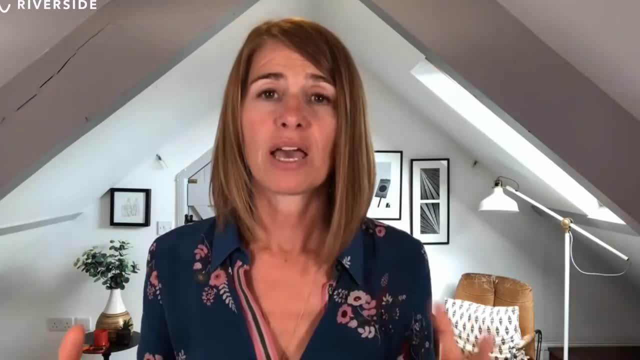 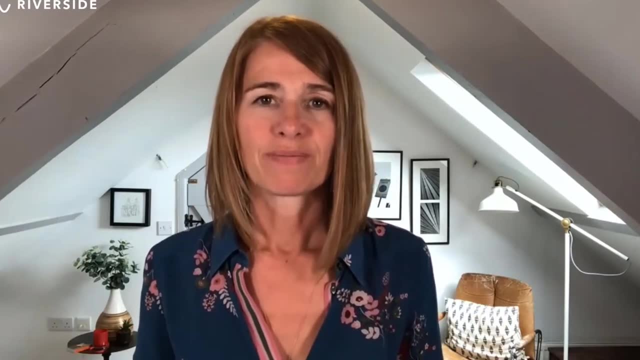 might make for social media, any videos you might make for teaching or for your websites. All of those points where people are interacting with you is where you're speaking. It's where you're showing up as a credible or not such a credible speaker. It's where they're making. 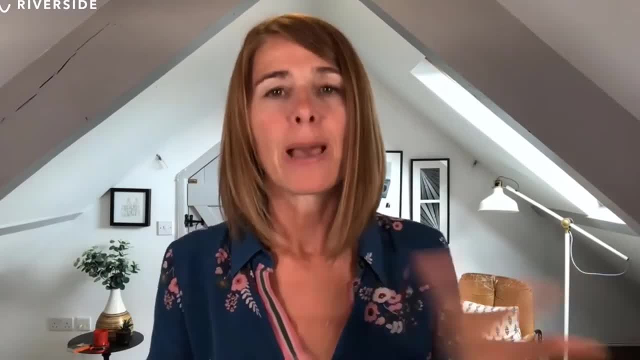 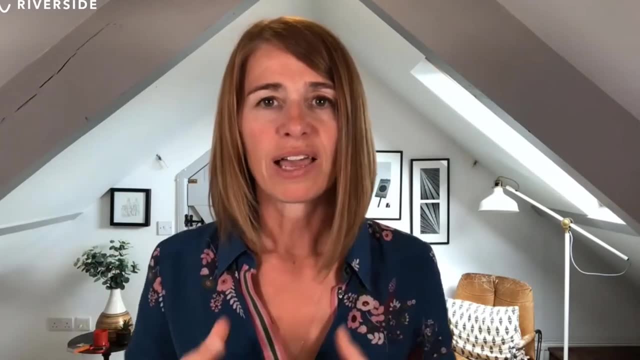 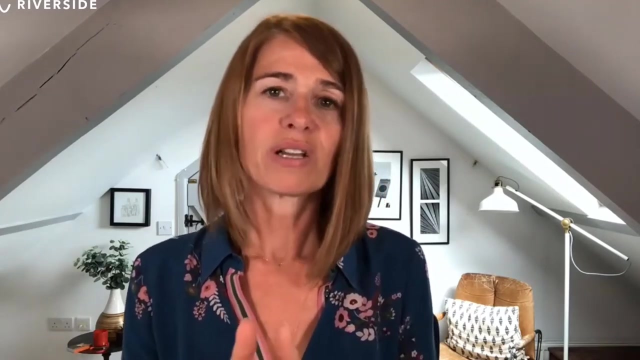 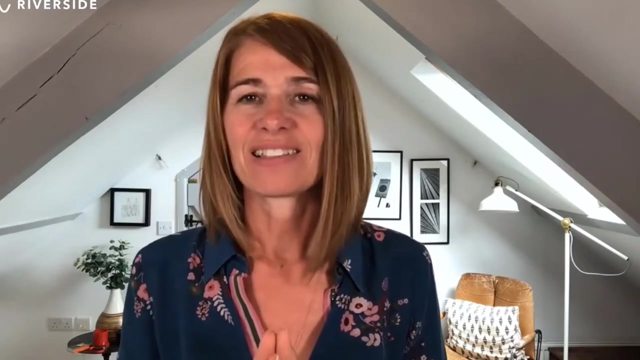 decisions about your competency, about your expertise, based on what they can see and hear on that video. So, in terms of entrepreneurial life, your credibility as a speaker is absolutely critical to the success of your product, your service or your business. Now, equally, in corporate life, it is exactly the same thing. 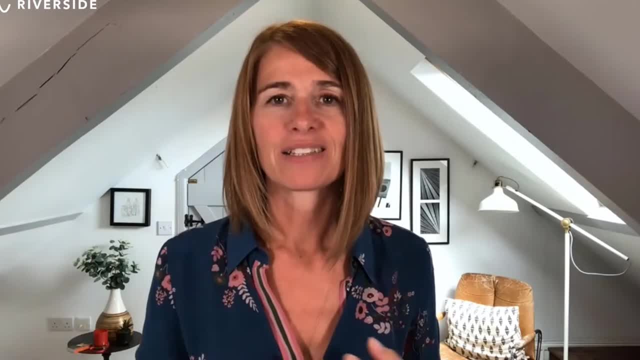 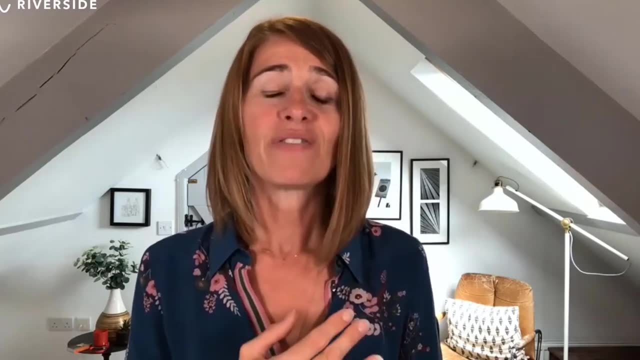 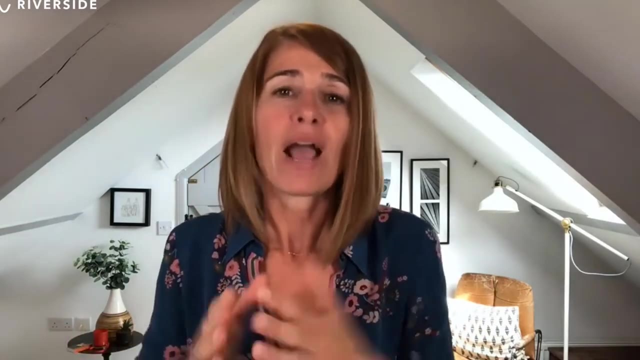 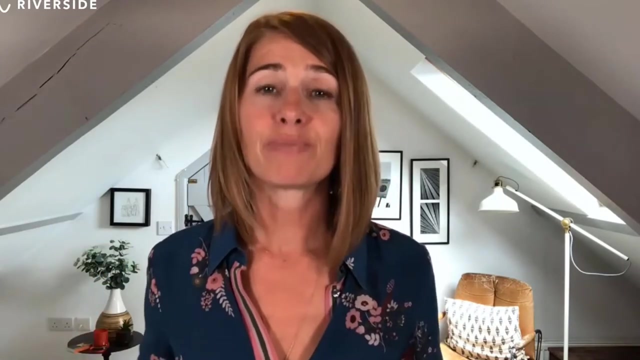 Those water cooler conversations, team updates, clients or supplier meetings, negotiations, interviews for promotions, even your end of year assessment. how you're doing all of that is how you pitch up, how you speak at all of those. The consistency with which you're credible creates the perception of how competent you are. 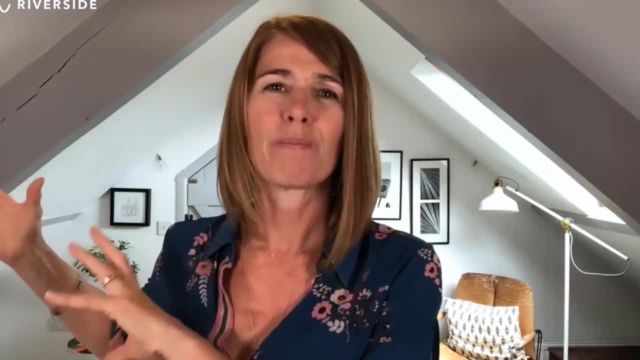 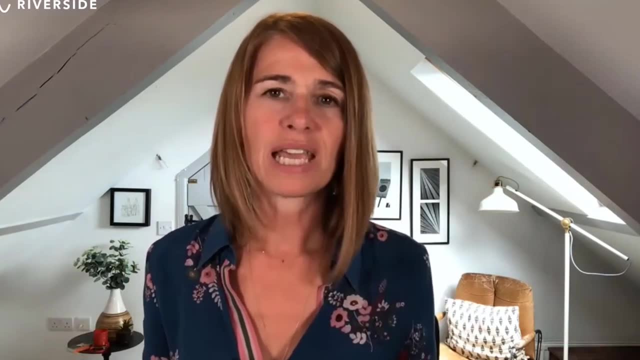 Now in a corporate space, you've also Got your work back catalogue, if you like to rely on, but often that can get put to one side and it's what people see and hear on a daily basis that they really take on board and that can become your story. 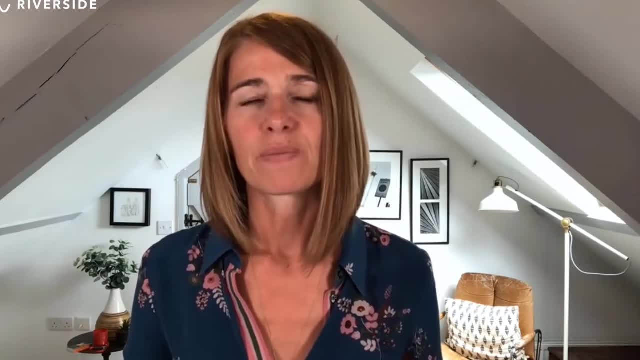 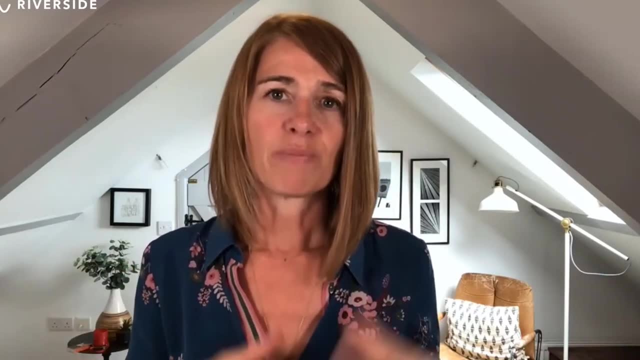 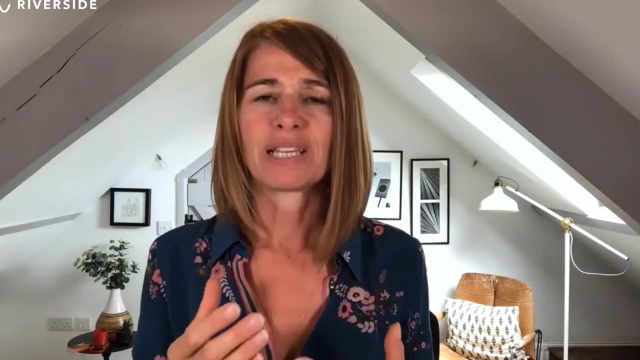 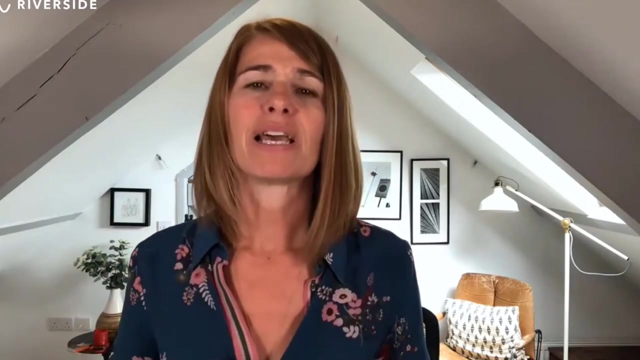 It becomes your narrative within an organisation. So being a credible speaker, whether you're an entrepreneur, whether you're in a corporate space, is really critical to business growth, to personal development, to your career development. And if you Have Haven't got that credibility, what I find is that careers, businesses are slightly stalled, they slow down, we can get a little bit stagnated for periods of time and they're not progressing in the way that we want. 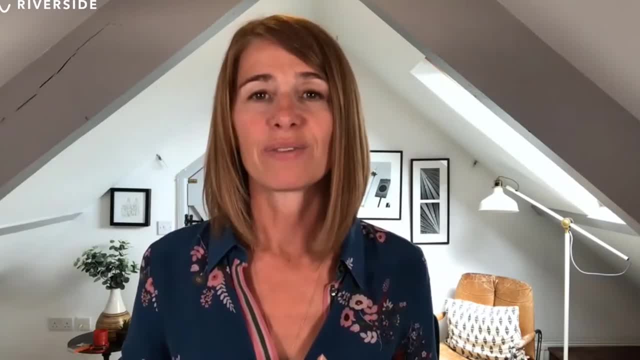 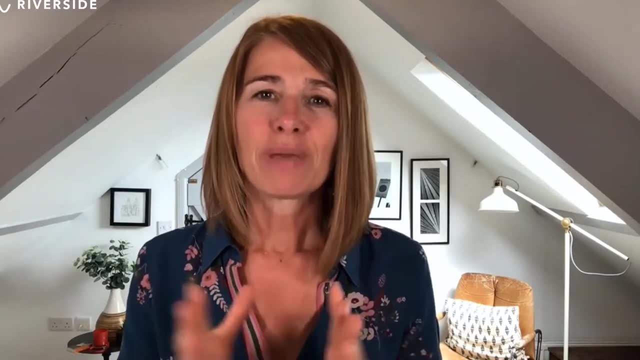 We're not being given the opportunities that we would really really love And we're all selling all the time. whether we think we are or not, we're always selling and people, as you know, will buy you well before they buy your idea. 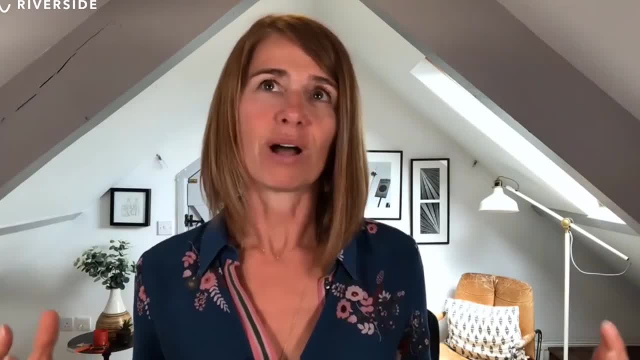 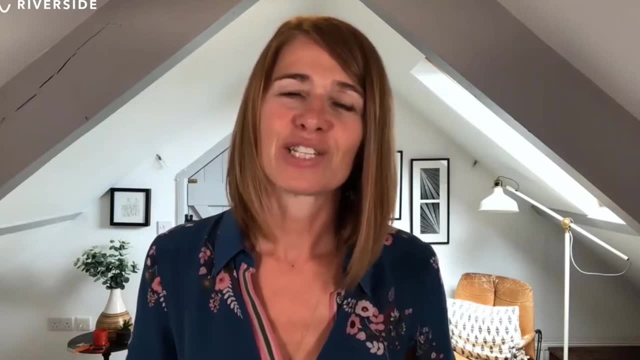 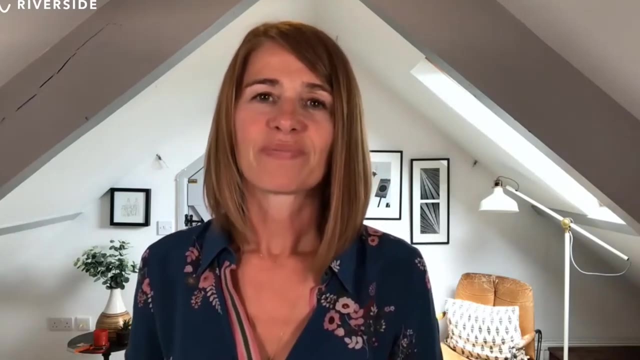 So being A credible speaker is an absolute, well, I would argue, a life skill rather than a business skill. So let's dive into those three building blocks. So we said they were pathos, ethos and logos, And pathos essentially means the emotional content. 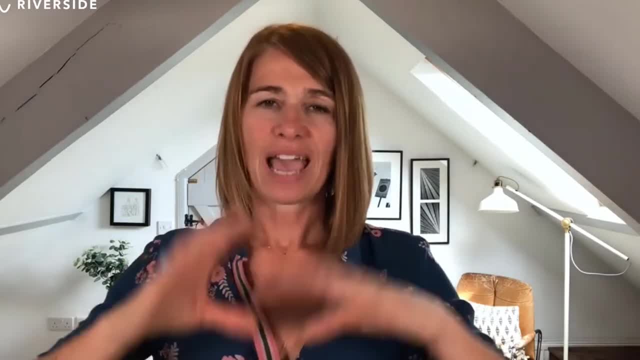 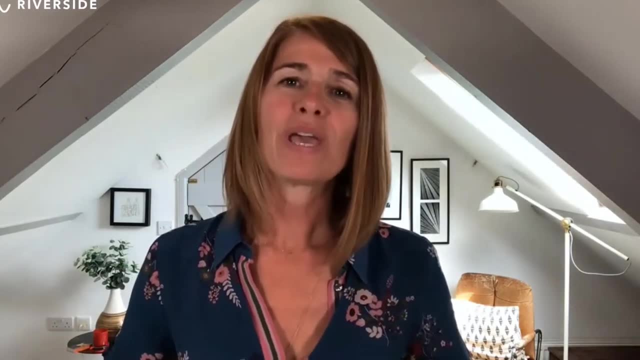 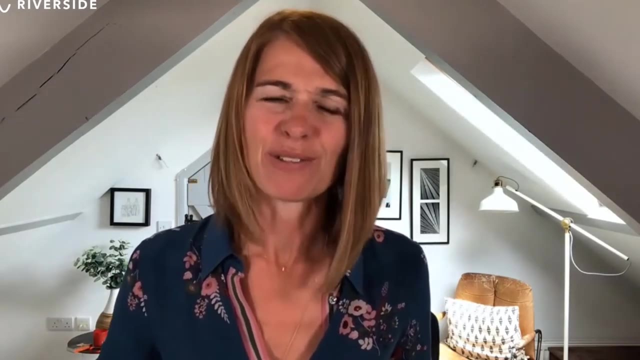 So, whenever you stand up to speak, we always want to be containing, have something that has Emotional content. We are, after all, human beings. Now, we love to kid ourselves that we make rational decisions. We don't. I know, you know that we don't. we make emotional decisions. 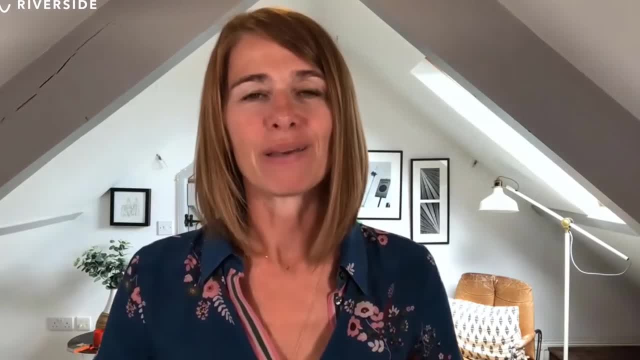 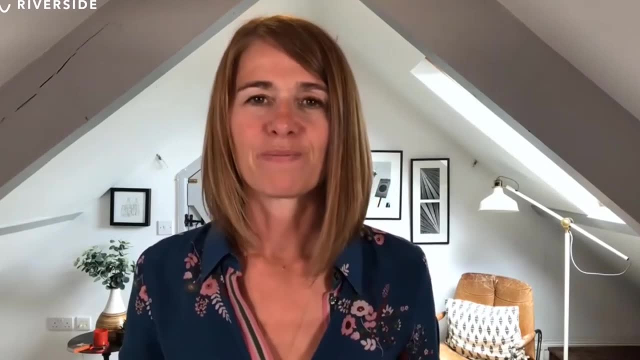 And then we find the statistics and the data to back up our emotional decision. Yeah, We rationalize after the fact to make sure that we feel good, that we've made the right decision. So whenever we speak, whenever we're updating, whenever we're presenting, 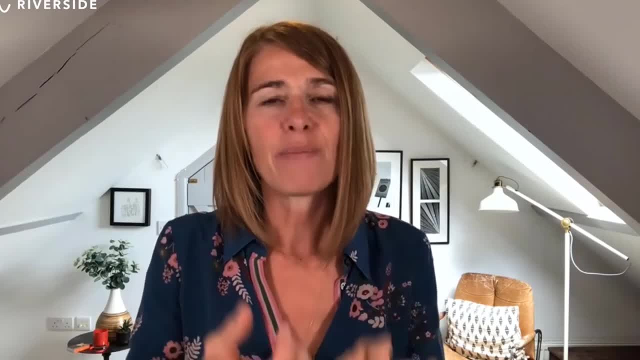 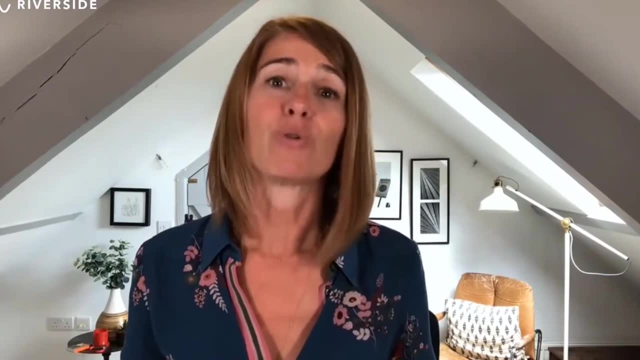 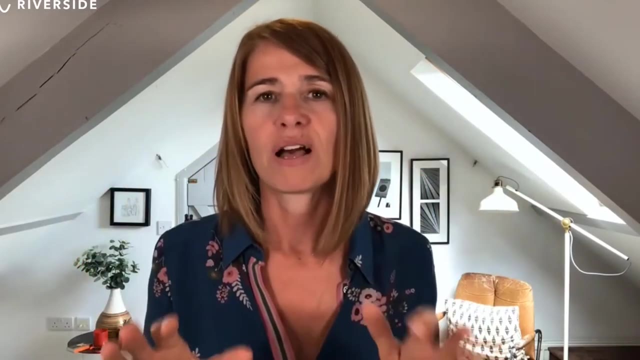 We're. whenever we're pitching, we always have to have some level of emotional content. If there's no emotional content, there's some very important things that happen or don't happen. So there's no emotional content, It becomes: you could present the most rational idea, the most rational solution. 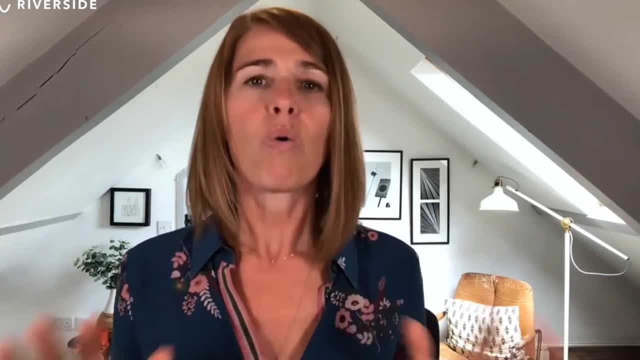 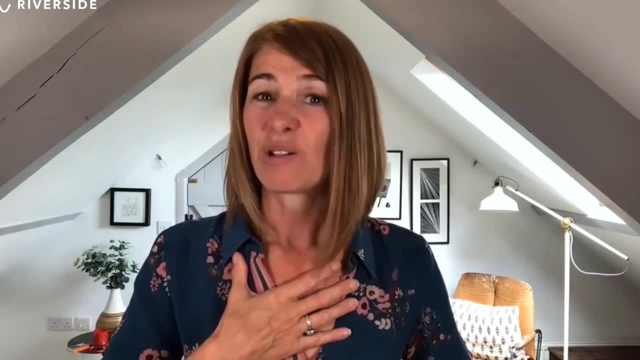 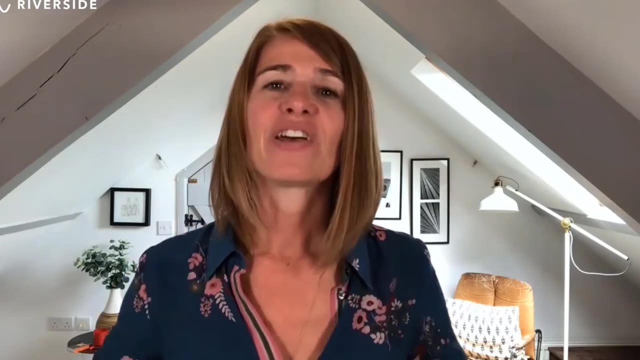 It's incredibly logical, It makes sense, It's inexpensive, All the things Right, It's ticking all the boxes. But if, as a listener, I don't care, Then I'm not going to take that action. And the way that I start to care is if there's an emotional content. 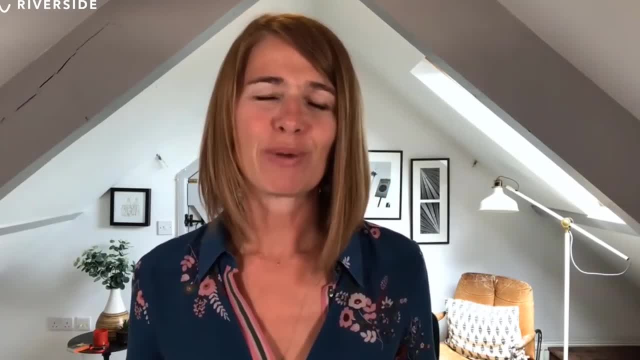 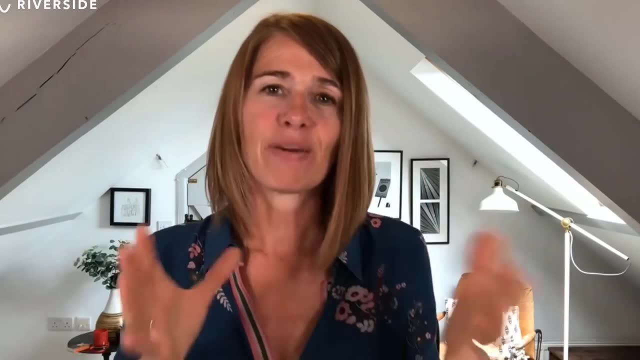 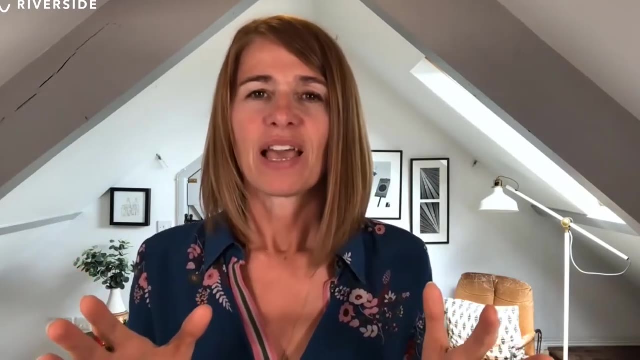 So I'm going to refer to an example. I've spoken about this before, but there was a firm that created a MRI machine- right, FMRI machine. It's incredibly complicated, Really really massively complicated physics, And this machine had incredible upgrades. 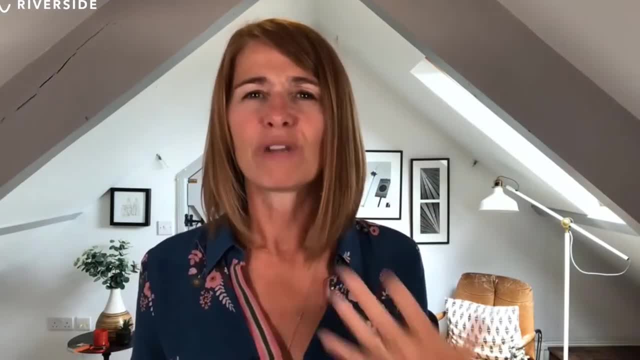 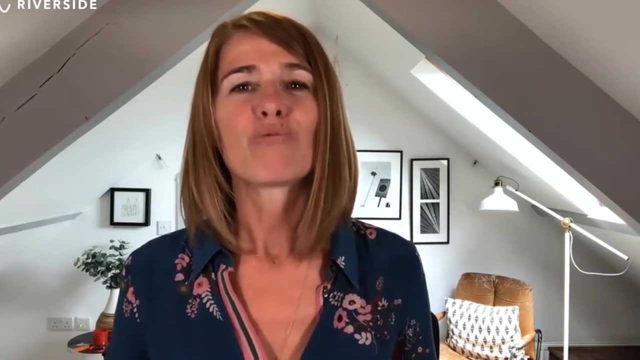 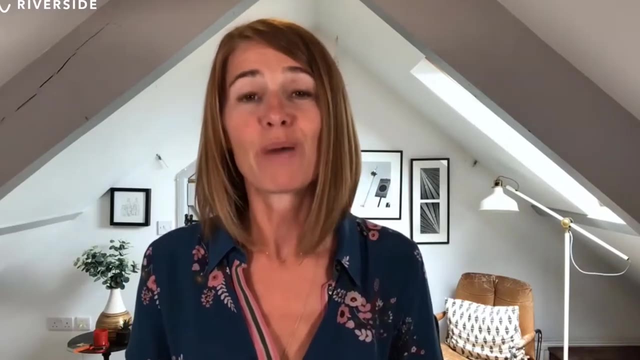 It did amazing things that were different and really powerful compared to its previous incarnation. Now the presenters luckily realized that standing on stage and telling a bunch of doctors and a bunch of purchase order people within a purchase departments within a hospital all about these new functions and features was going to send them to sleep. 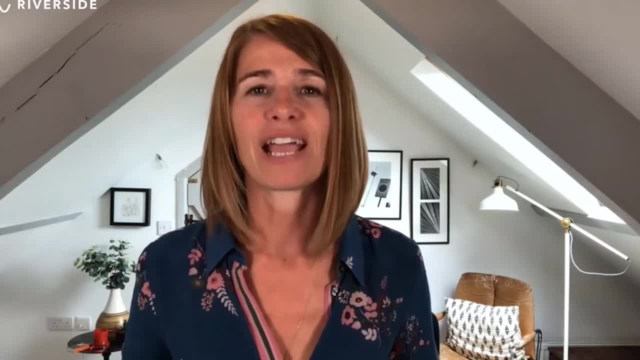 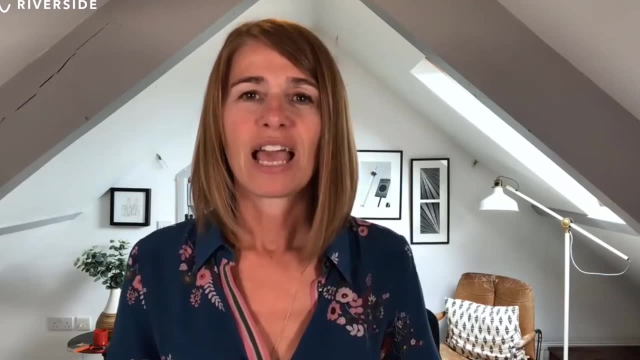 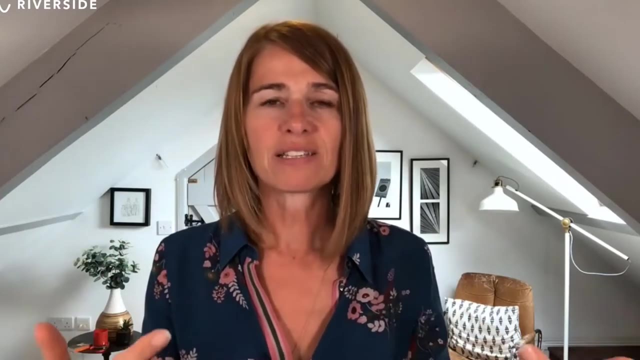 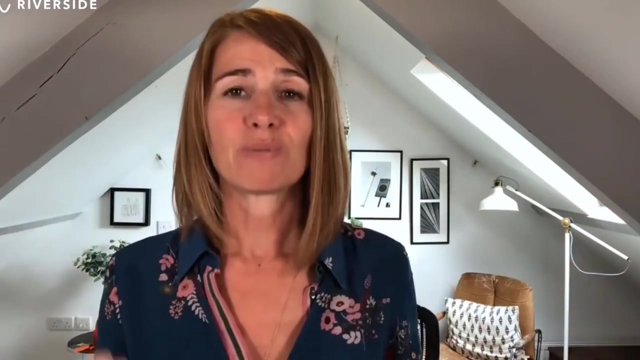 And they just didn't, They just didn't care. So they very cleverly created Lisa and David. and Lisa and David were two patients who were going to be scanned through this machine And they told the story of Lisa's journey through the machine and David's journey through the machine and through their illnesses and how the machine was going to help diagnose and get the right treatment for these particular individuals. 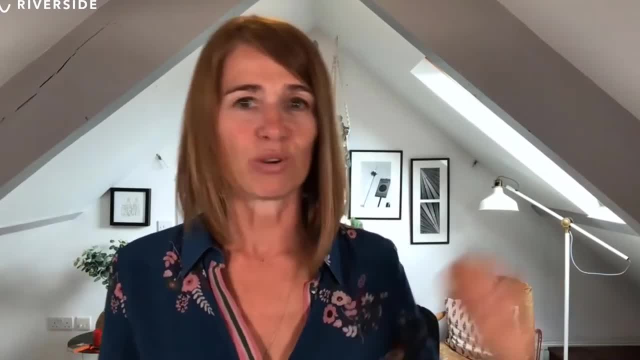 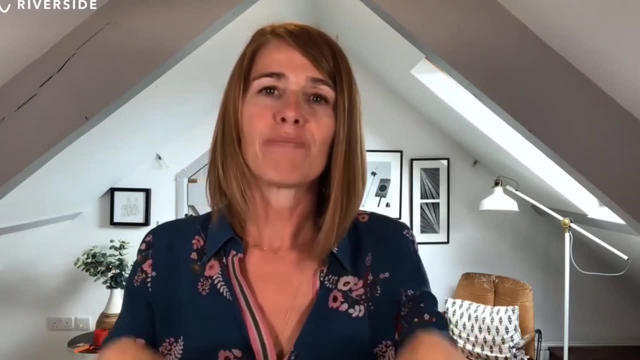 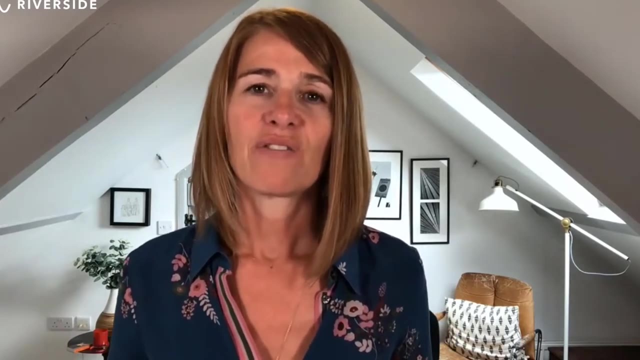 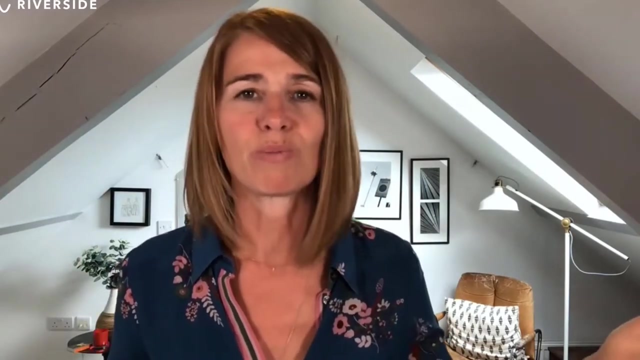 So the audience learned about what this new machine could do, What This previous incarnation couldn't do, through the lens of the patients, the end users, the people that would actually benefit from the machine. And that was much, much more moving, much more emotionally engaging for the audience than listening to a bunch of data about how the new functionality of this machine was so much more superior than the previous one. 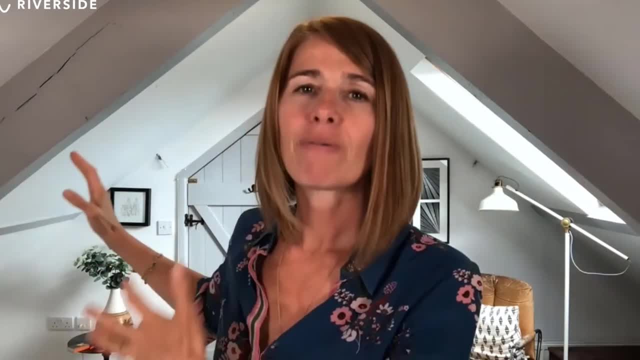 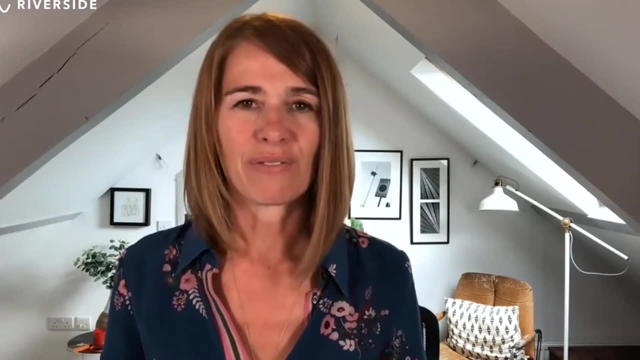 It was also so much more memorable because you could go away and think about and remember Lisa and David and their stories, And then you could think about the data. You wouldn't remember that when you left the room, You'd just be thinking about the price. 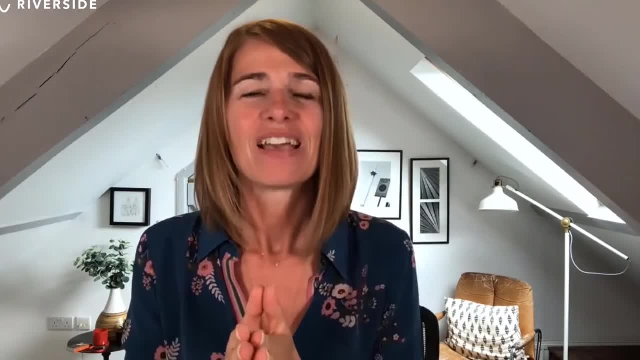 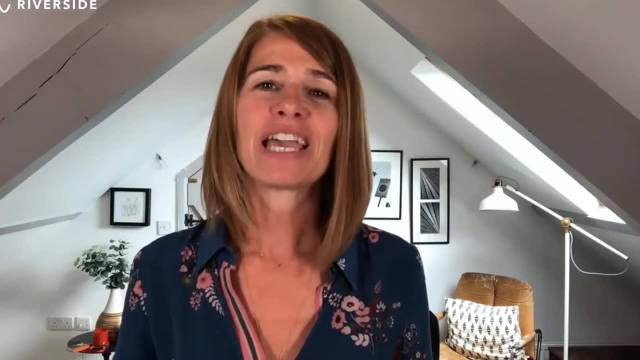 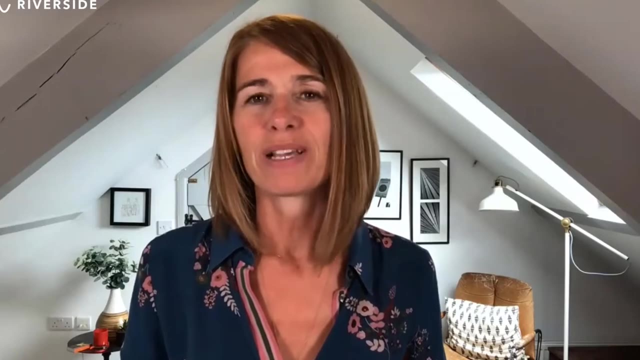 Almost certainly not cheap machines. So we want emotional content, and that can come in the form of stories like Lisa and David. It can come in the form of anecdotes or testimonials. It can come in the form of sensory language. So what do I mean by sensory language? 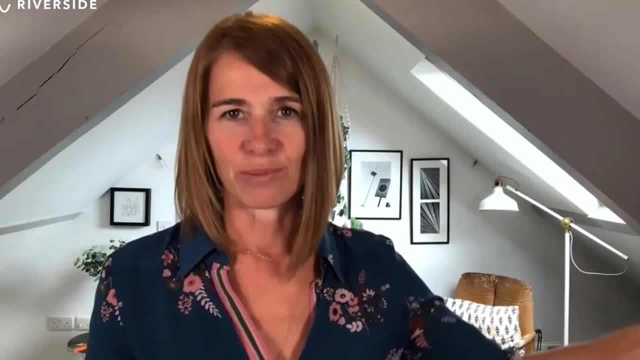 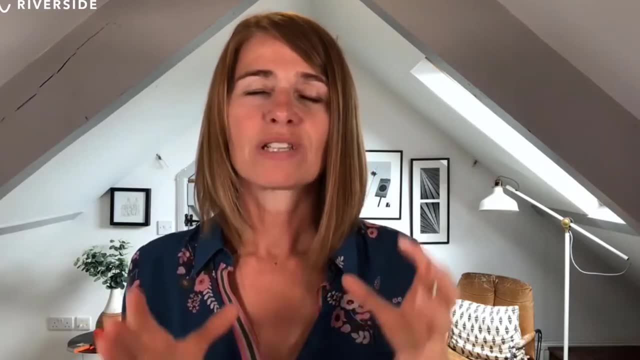 So I could say something like: last Tuesday I took my test, I took my daughter to school. Or I could say: it was Tuesday, The rain was coming down in buckets, It was freezing And we both realized that our waterproof coats were no longer waterproof. 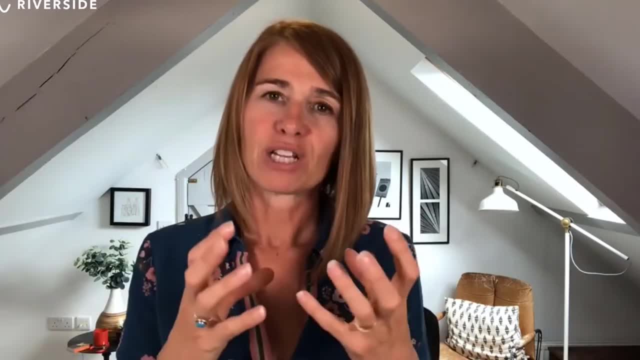 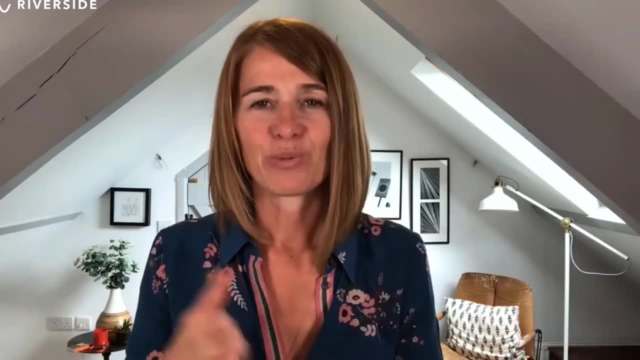 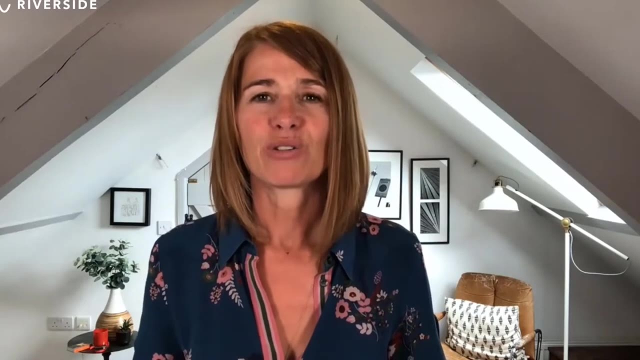 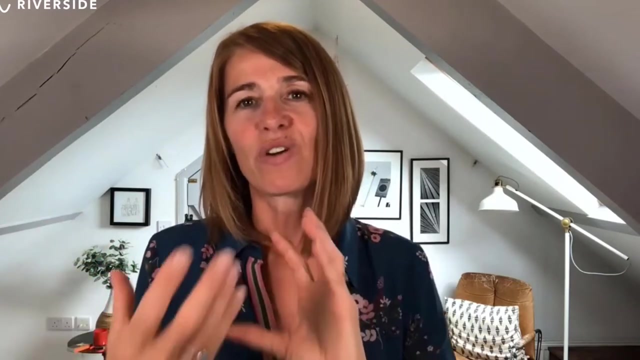 So you can see that by using that sensory language you've got a much more visceral sense of time and place. So the more sensory language we can put into our content, the more it becomes alive in the minds of our listeners. So we really want to be making sure that we have stories, emotional content, sensory language to make sure that it feels very human to the other person. 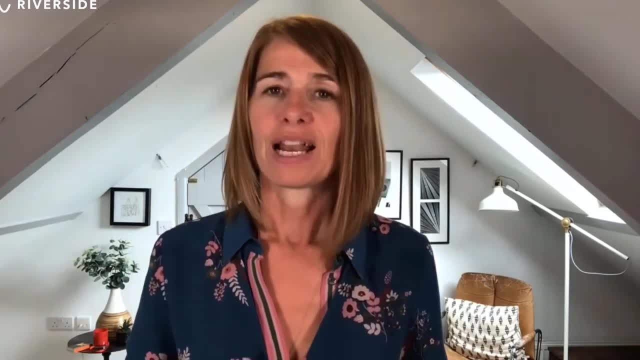 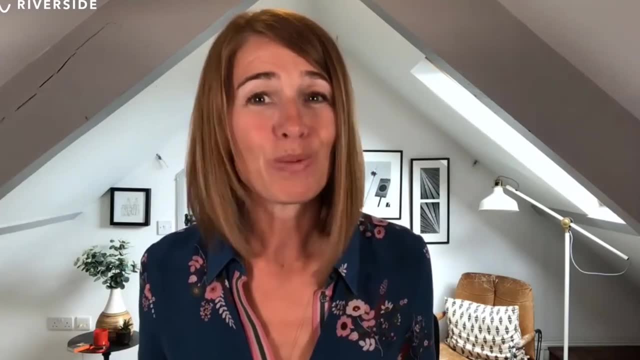 You can also do two other things. One: you can use humor, And I'm going to caveat here: not jokes. Unless you're a stand-up comedian, please don't use jokes, They don't work. You can use humor, though. 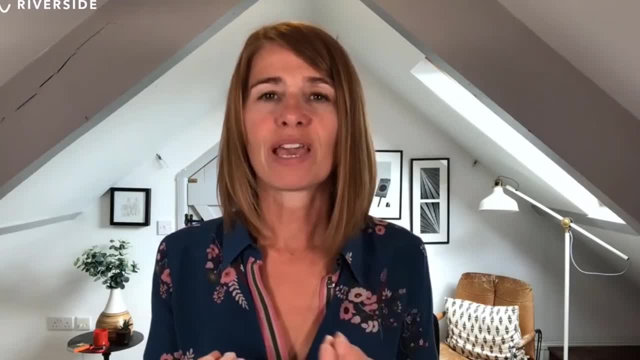 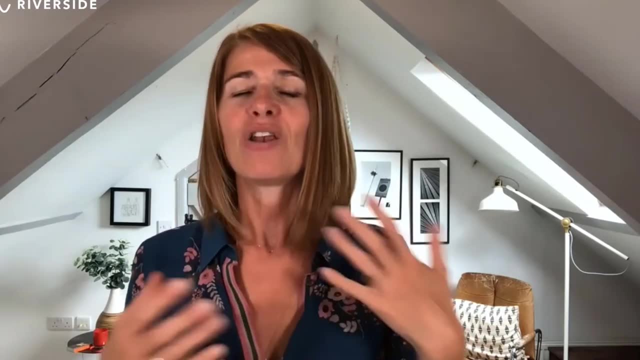 And you can use fundamental truth. So fundamental truth is something whereby you and I both know how annoying that thing is. So say, you come home from work, you've had a long day and all you can think about is making yourself a nice cup of tea, and you go to the fridge and there's no milk. 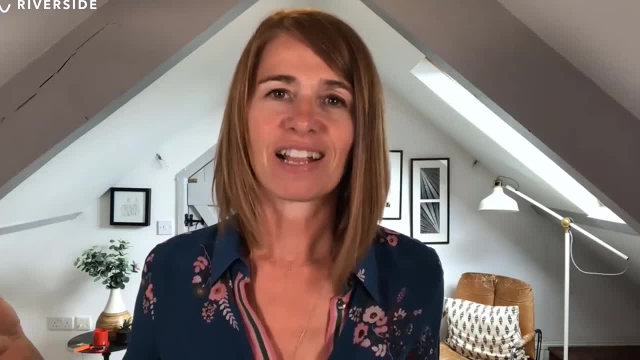 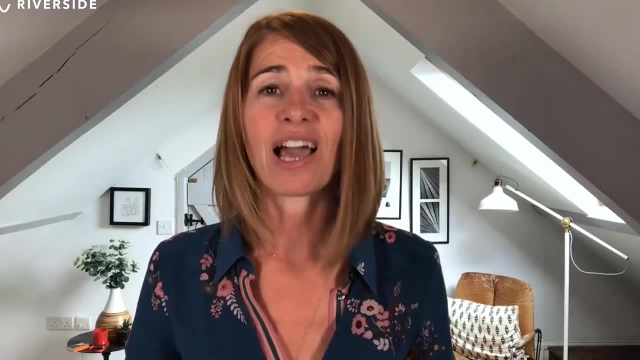 Someone's put the empty milk bottle back but it's there's nothing in it Right Now. you know- I know everybody that we know that has a fridge has probably experienced that at some point in their lives And you know the kind of like oh, feeling of that moment. It's a fundamental truth. 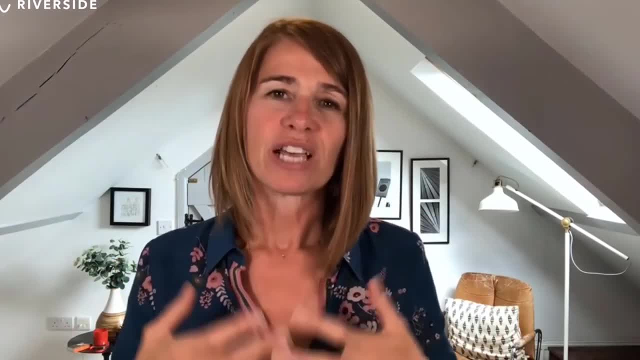 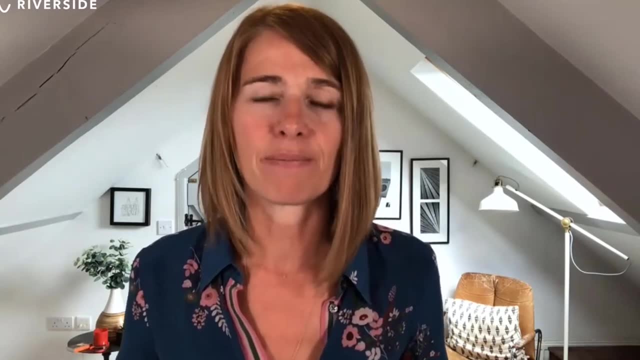 So, just like falling in love, it's a fundamental truth. So if you can use something that other human beings, or most of the human beings that you're likely to be talking to, will have experienced at some point, then that's creating an emotional connection with your audience. 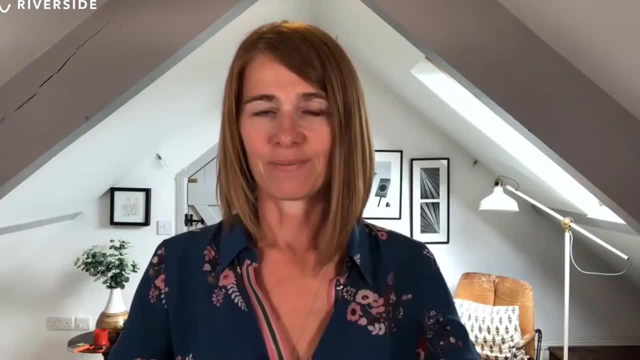 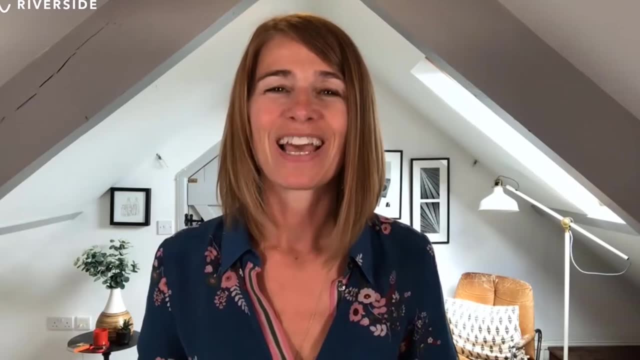 So if you can do those things, people start to care. If they start to care, they're emotionally engaged Right. You've got their attention Super, super important. Also, they're far more likely to take the action that you're asking them to take. 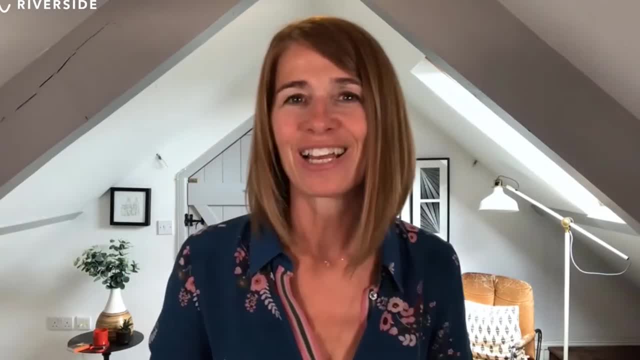 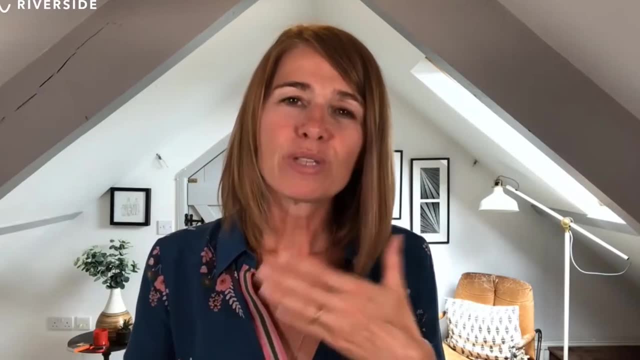 So that could be continue the conversation. It could be sign on the dotted line, It could be introduce me to this person or that person, Give me the promotion, whatever it might be. So we always want to be engaging with the other person so that they are moved along in the conversation. 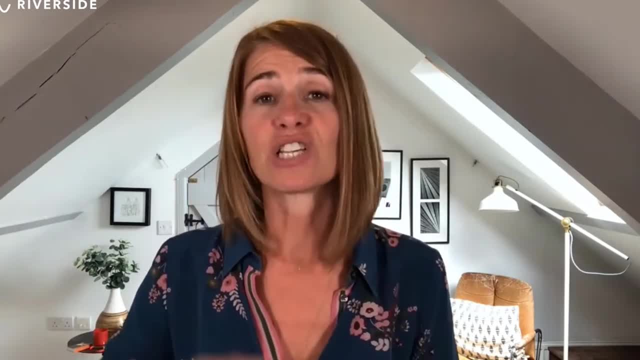 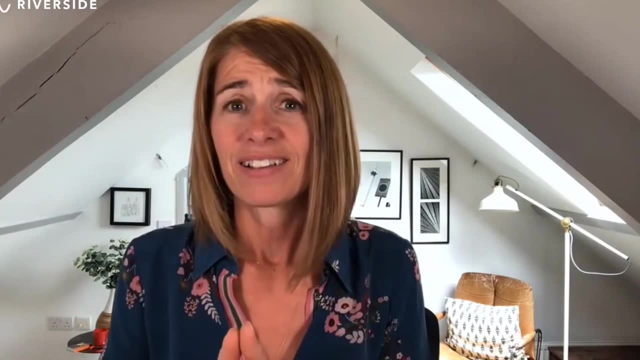 And they're much more likely to say yes to continue this conversation or yes to an actual idea, So very, very important. If it's not there, then I'm not likely to be engaged. So I might stop listening, I might start thinking about what I need. 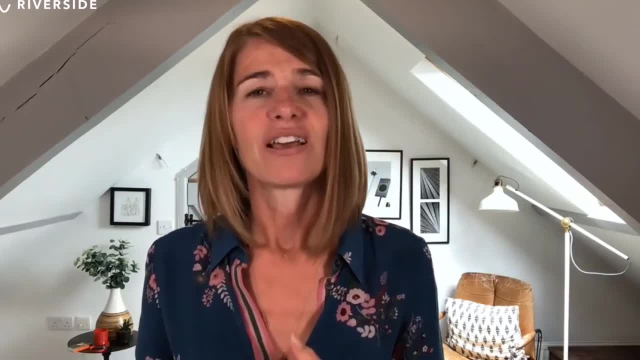 I might start thinking about what I need to get in the shop later that day, or what am I going to have for lunch. So I'm not really listening to you and I'm not engaged, So I'm probably not going to take the action that you're asking me to take. 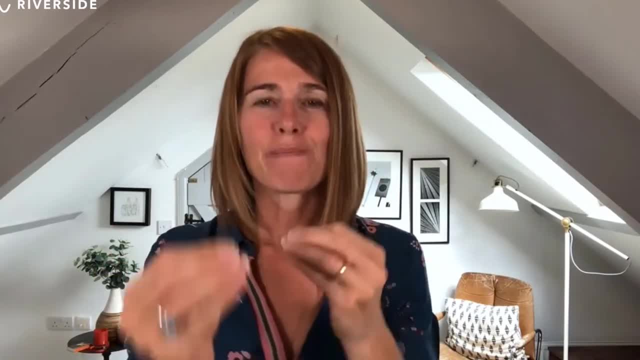 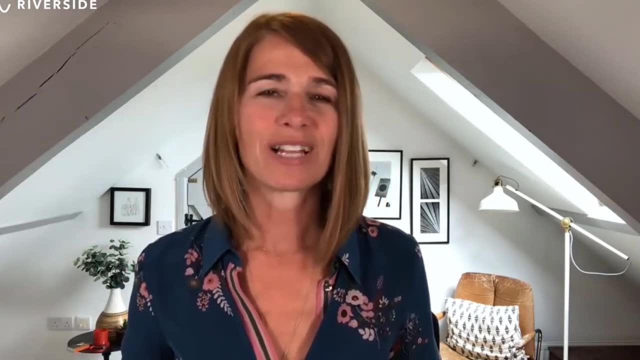 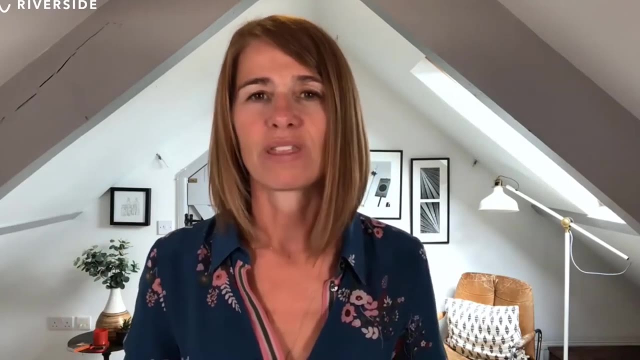 So very important that we create an engaged emotional connection with the other person. So ask yourself, when you do stand up to speak, when you are presenting or pitching, are you good at creating that emotional content, that emotional connection with your audience? Yes, 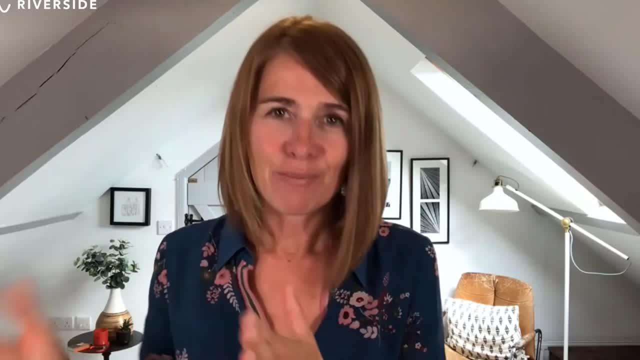 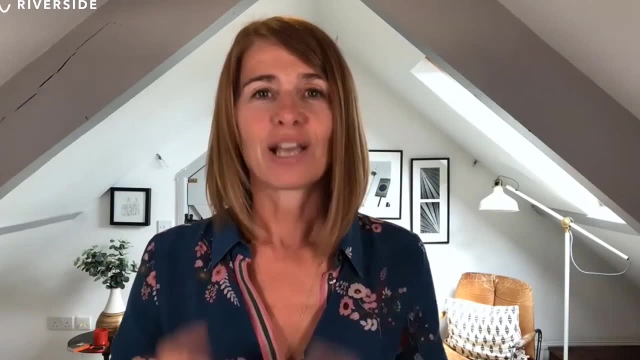 And if not, what could you do To make that, to make sure that that's always there, that's always part of your presentation or pitch or conversation? So that's pathos. Let's move on to logos. Logos essentially means logic. 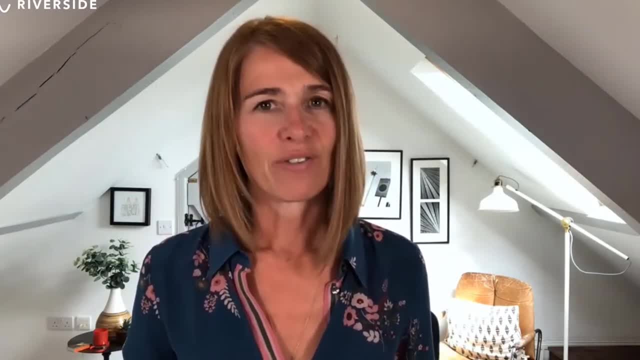 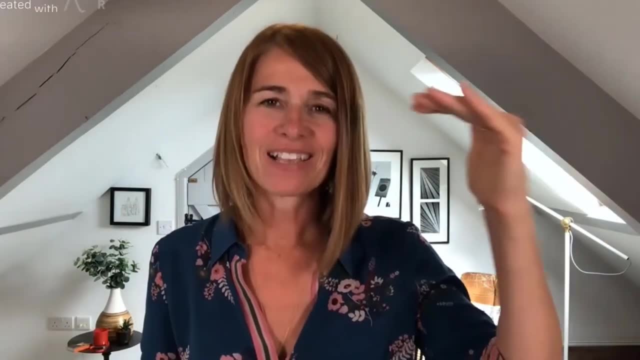 So here we're going to be looking at the logic and the flow of your argument. So does your argument, and I don't mean fighting or conflict, but does your argument make sense from the beginning to the end? Is there a logical flow? Do I know where I'm going? 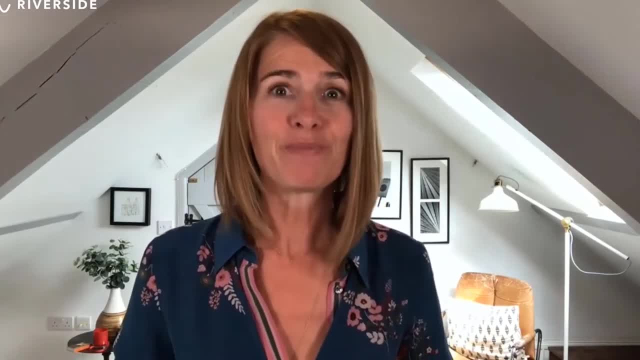 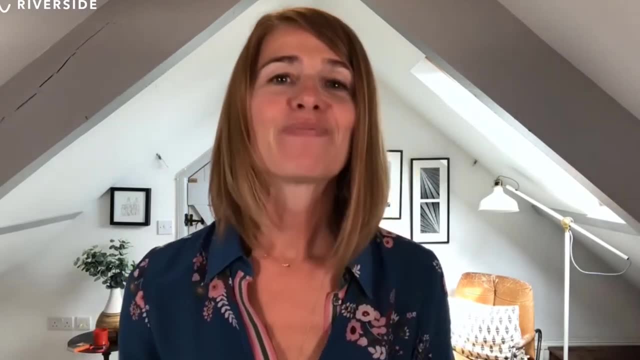 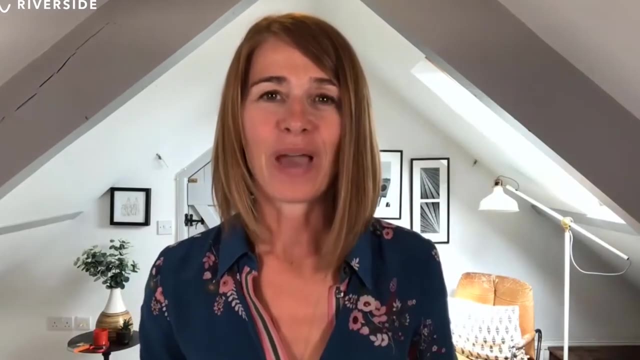 Now, sometimes it can be really helpful for audiences to let them: oh, didn't turn my notifications off. Sometimes it can be really helpful. Let me just do that now So it doesn't ping again. Um, sometimes it can be super helpful to let your audience know where you're going from beginning to end. 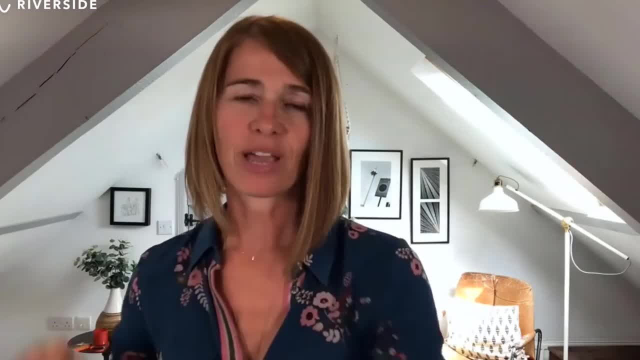 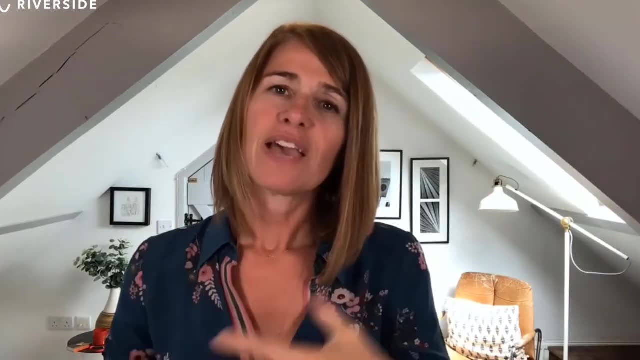 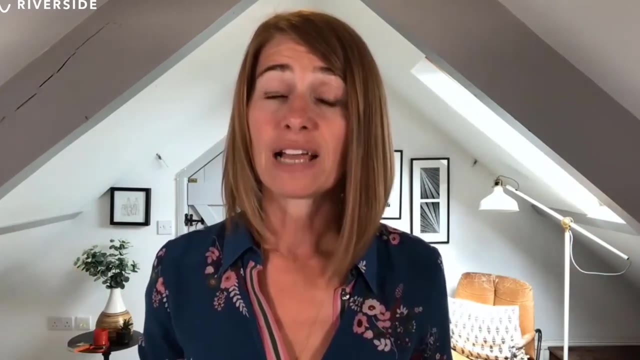 So we're going to go here, We're going to talk about this, we're going to talk about that, Then we're going to go over here. So sometimes it can be really helpful to notify your audience Where they're going. then you want to know that. if audiences don't know where they're going or there doesn't seem to be any plan to your conversation, they can feel really untethered and unsafe. 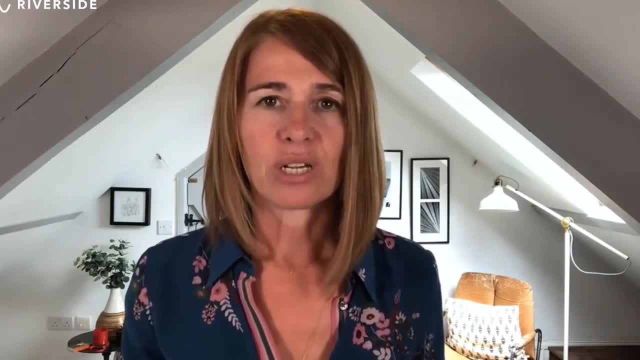 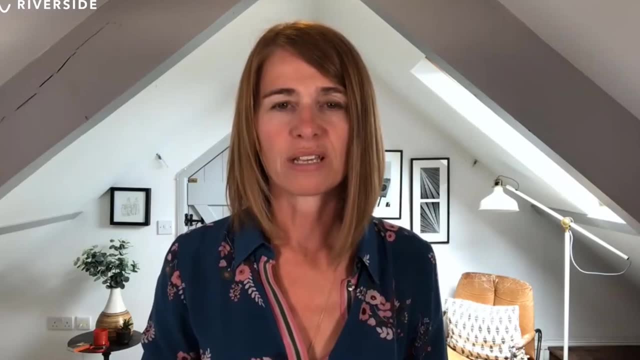 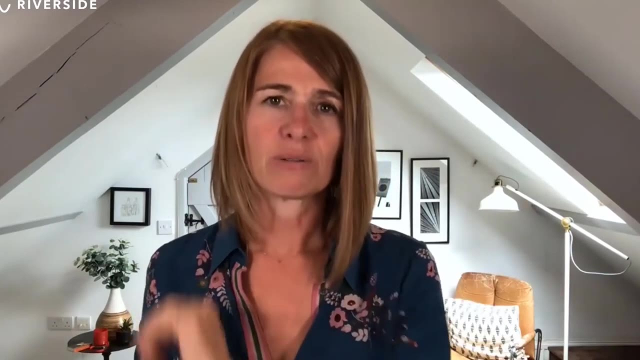 And it can feel like they don't know what they need to do next or where they're going, And that can make them feel really unsettled And it means they stop listening to your content. So sometimes it's as simple as just letting people know where you're going in your conversation and then making sure you stick to that. 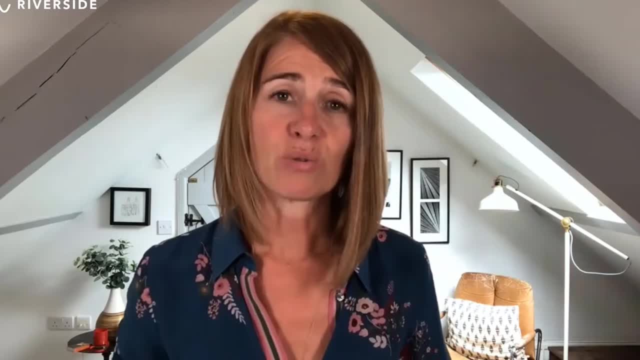 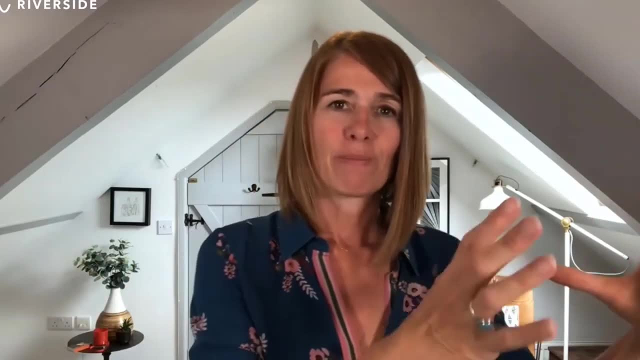 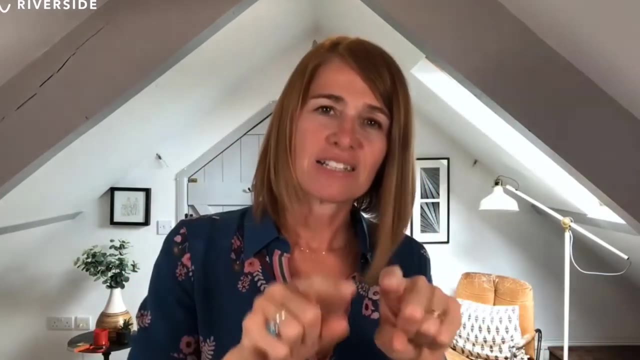 Process that you're talking in the ways that you've said you're going to talk. Sometimes it's about building coherence, So having the building blocks understanding block a, because before you went you need to understand block a before I can introduce concept B, and then you really need to understand concept B before I build on and understand concept C. 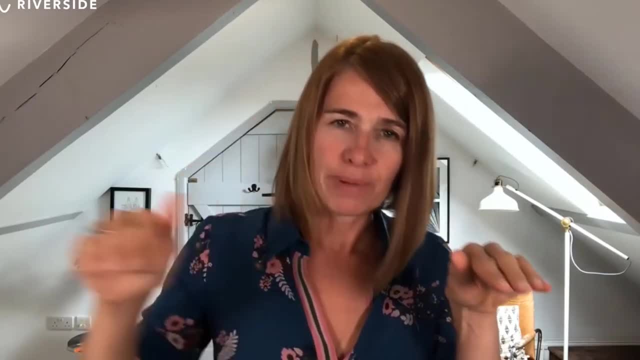 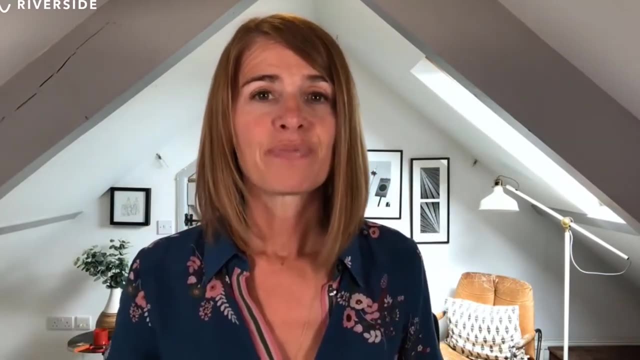 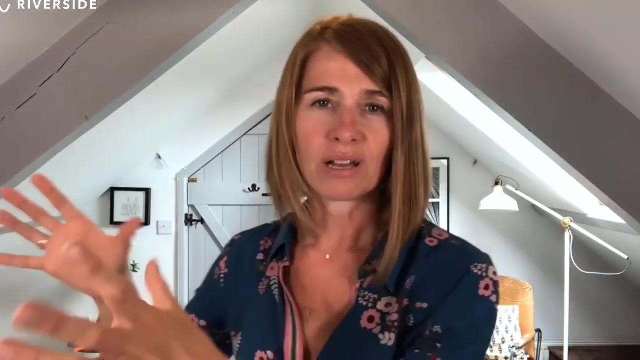 So very important that we are building that coherence, building those building blocks throughout your presentation. If there's complex information That People really, really need to understand, So sometimes it's about that. It's also about data and evidence. So if we've told our beautiful story, so let's go back to that idea about Lisa and David in their MRI machine. 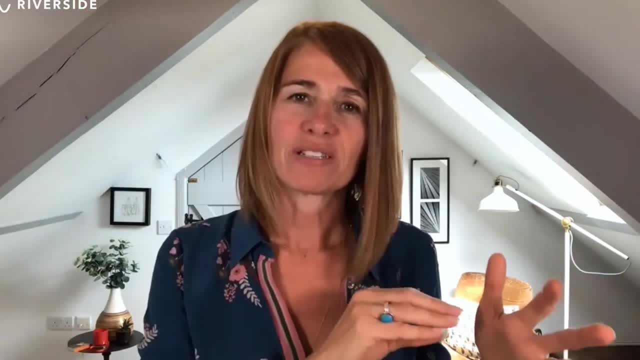 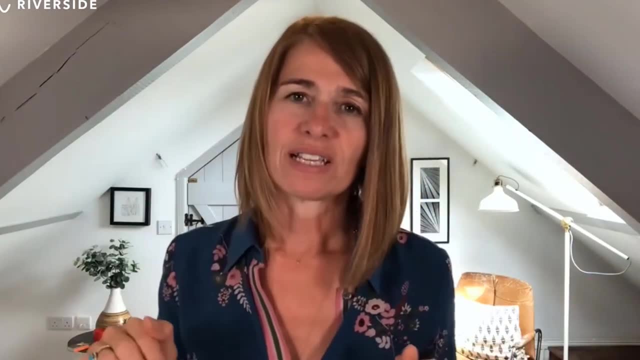 Now I need to support those stories with evidence, And I can do that at the same time, I can do that following or I can do that separately. but I need to show the evidence that it didn't just work for Lisa, but it's worked for, you know, 3000 patients who also had similar conditions. 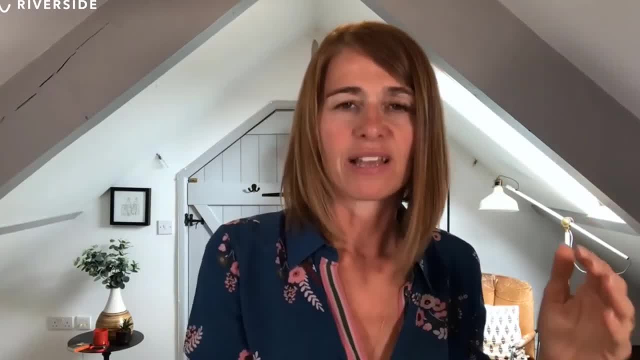 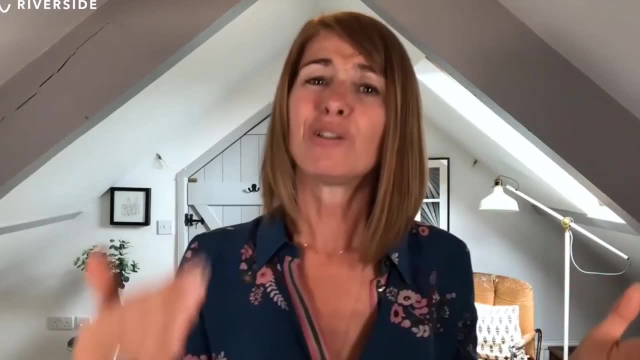 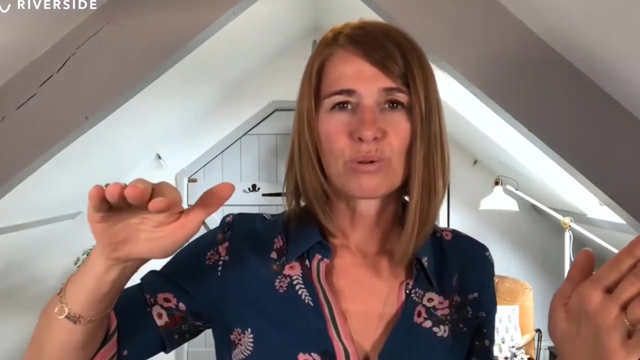 To Lisa and we had this much success rate that the people were diagnosed correctly. there were no misdiagnoses. there were no. there were limited amounts of people who were included in the diagnosis, who actually were fine, So it's really important that that data is there to support the story. 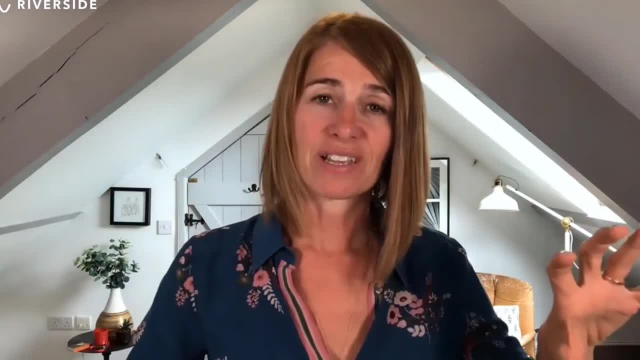 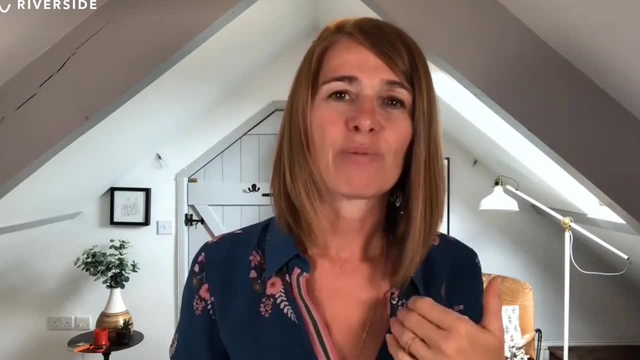 Remember what I said. you know you make that emotional decision and then you look for the evidence. So we need to have both, not just one or the other. If you give me all the data, as I said, I will probably buy in. 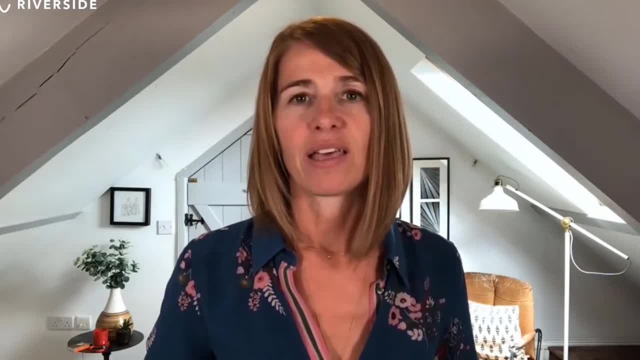 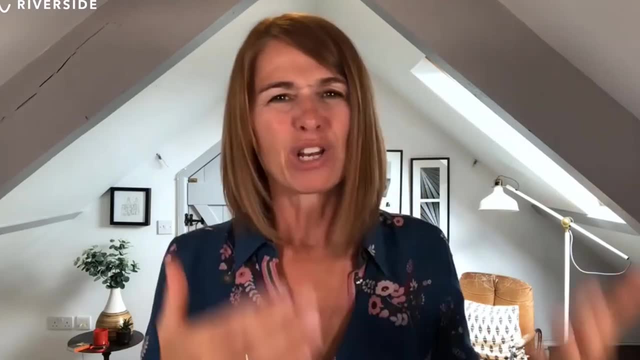 So I'm going to listen to it in a kind of like: oh yeah, well, that makes sense kind of way, but you haven't, you haven't caught my heart, I don't care. so I'm going to kind of listen and I'll consider, but- and it might look right on paper, but I'm not just not really in it. 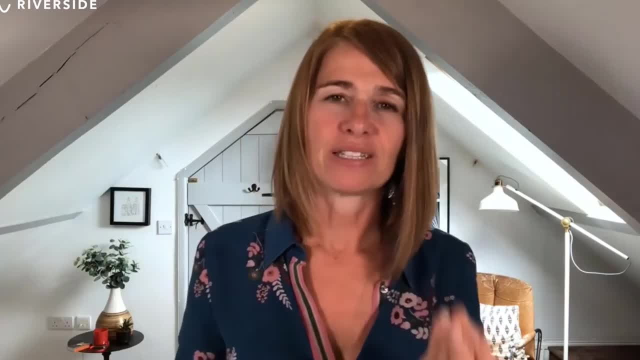 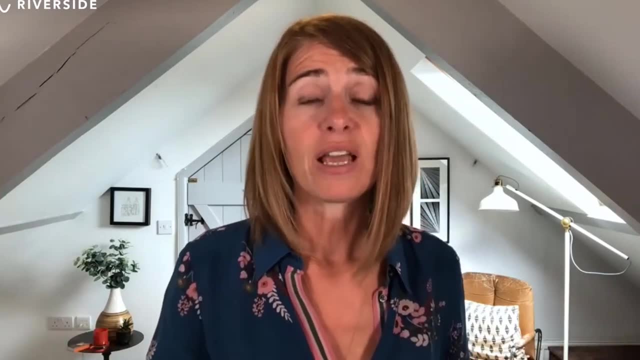 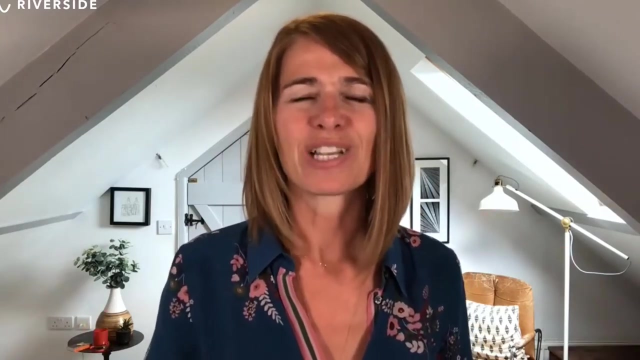 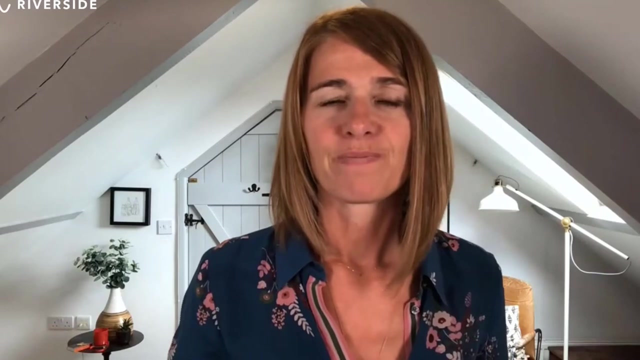 Yeah, So we need to have both. We need the emotional connection, and then we need the data and the evidence to support. Now. that data and evidence could be hard data, like in the fMRI machine, or it could be anecdotal, It could be testimonials, it could be um, it could be client success stories, it could be all kinds of things, but we need some evidence that what you're talking about genuinely makes a difference. 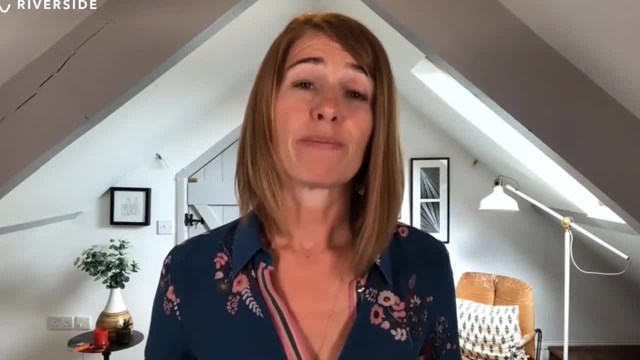 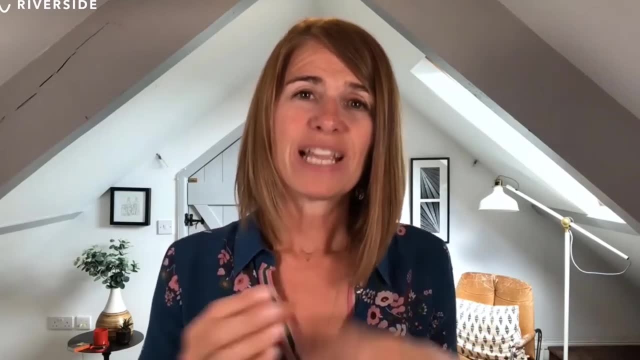 So we need that there. Now the other thing that is quite important here- and not in all conversations, but often in most business conversations- we need to have a kind of end point. So there needs to be a call to action. So what needs to happen next? 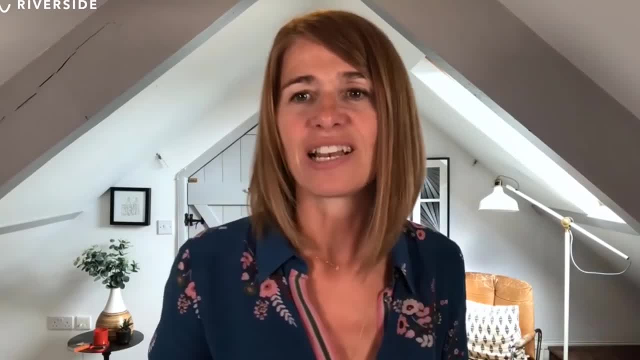 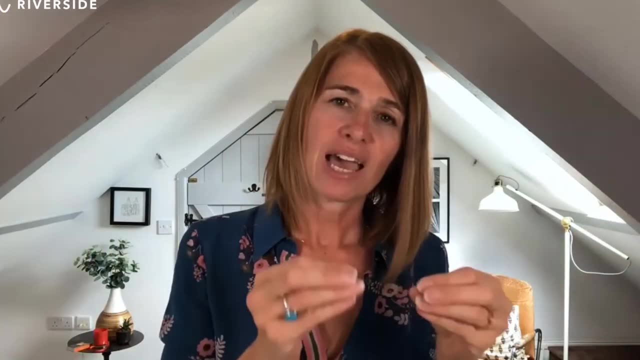 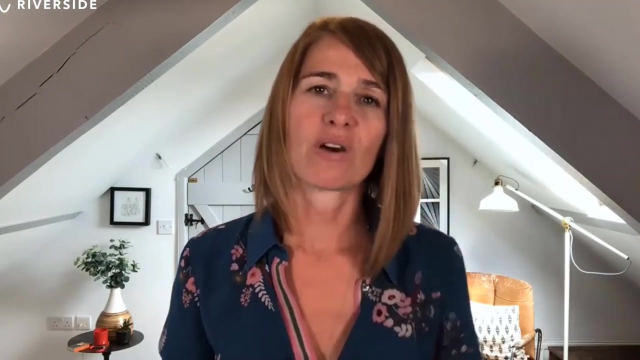 And that might be as simple as Uh another meeting to get a discussion in, let's uh, get a signature, let's agree on this budget, Let's uh whatever it might be. but we need to have some kind of end point where we're pulling it all together in a logical way that is moving the conversation onwards. 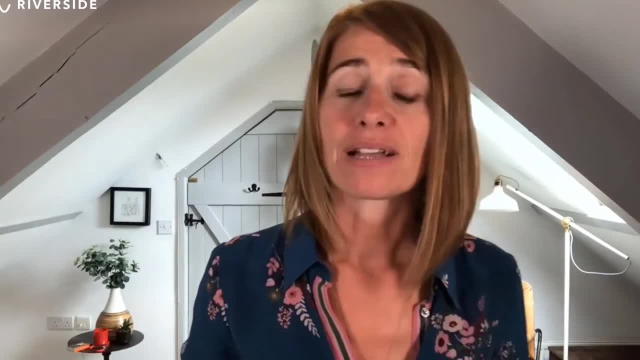 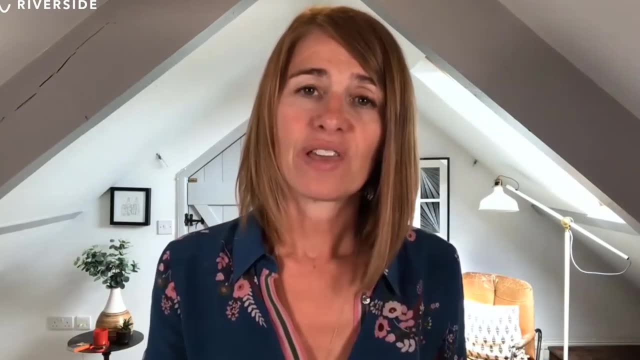 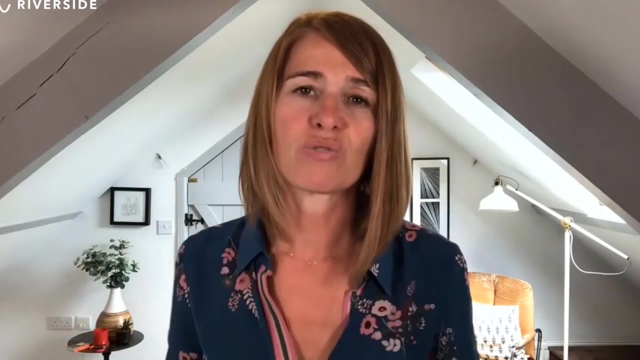 If we sort of let it drift, at the end all that impact starts to leach away. So really important that our listeners feel that we are well researched, That we're credible, that we are presenting strong data to support our strong emotional content- uh, so that it looks and feels robust. 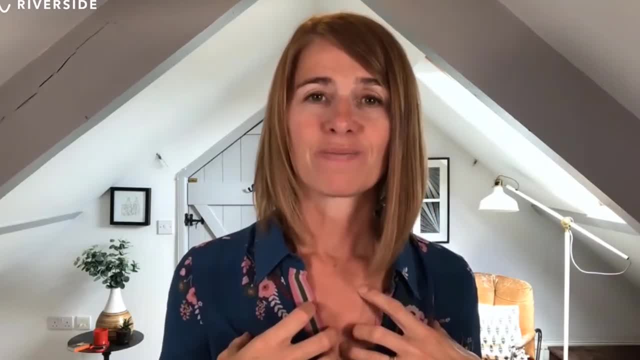 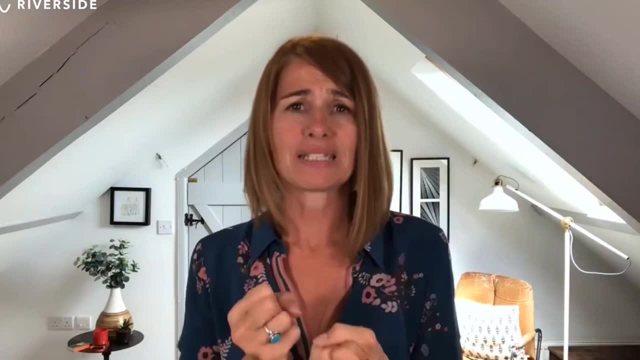 And then we are perceived as robust. Now, equally, if it's missing, it can be very confusing for your audience. If there's no structure, they don't know where they're going And they feel a little bit unsafe, untethered. stop listening. 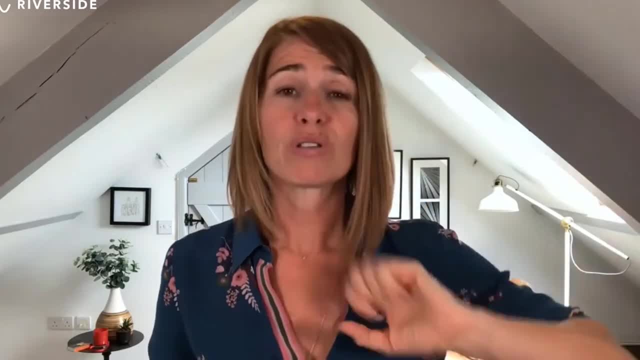 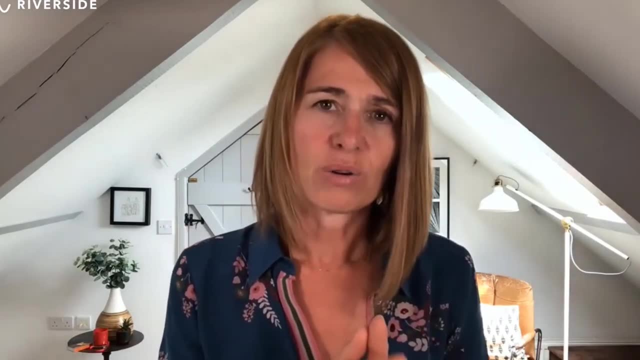 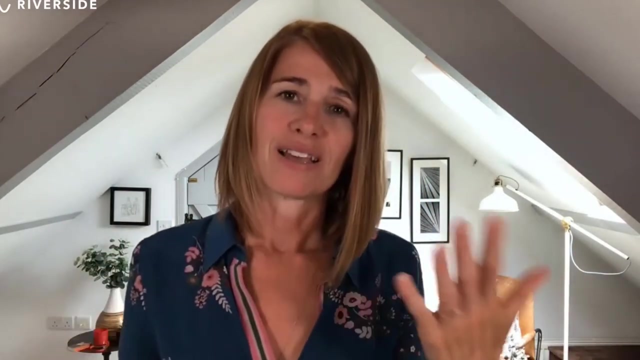 They're not necessarily engaged, or if we bamboozle them with too much data, they sort of blink A bit and then they start to switch off. either way, we've lost our audience. So we really want to be making sure that we keep them with us, with the right balance of emotional content and data and logical argument to support our ideas. 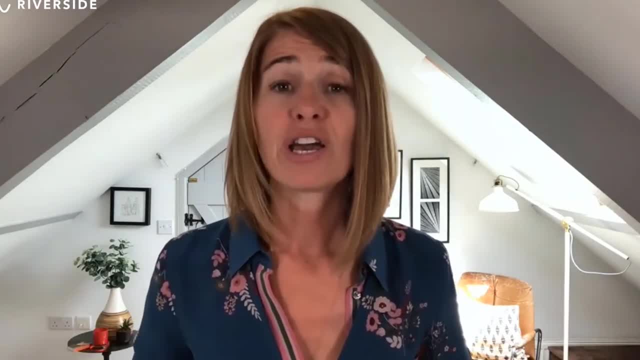 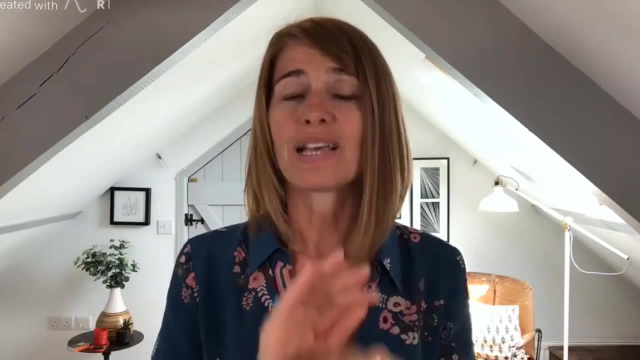 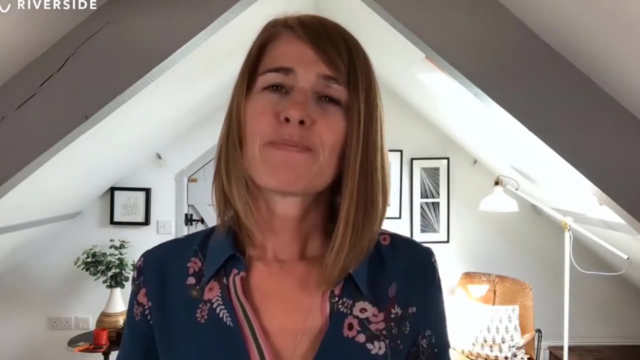 So those are two of the main building blocks. Now the third one is absolutely critical, And I would say that most people do think in some ways about those first two blocks, Uh, and then they perfect their decks, They think about what they're going to say. um, this next bit, this third block, I would say, is the block that gets missed the most. 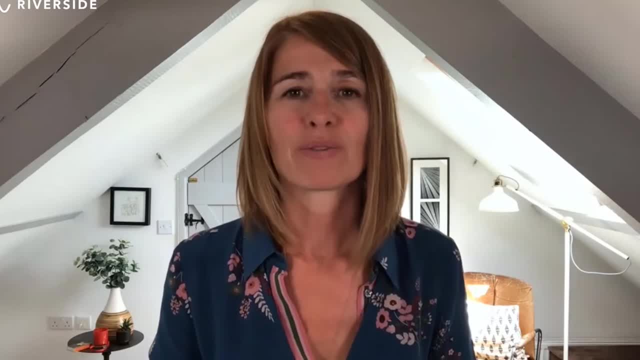 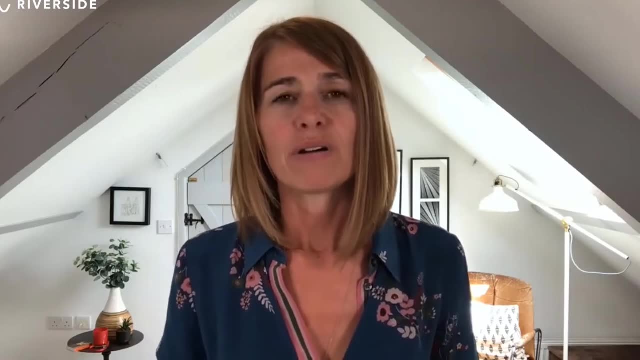 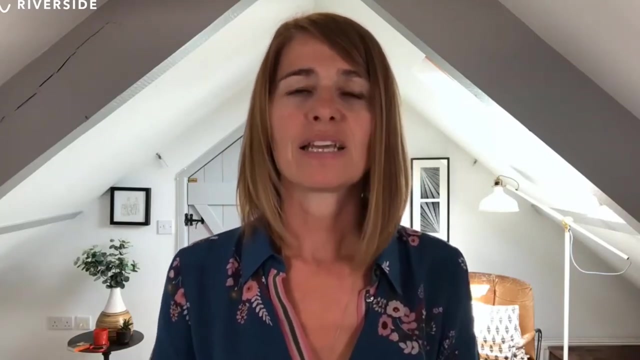 This is how we're going to say it. So this is really about um credibility. It's the ethos bit of the triangle. Now, Aristotle thought about this in two ways. He thought about, lived in ethos, So lived in credibility and ethos in the moment. 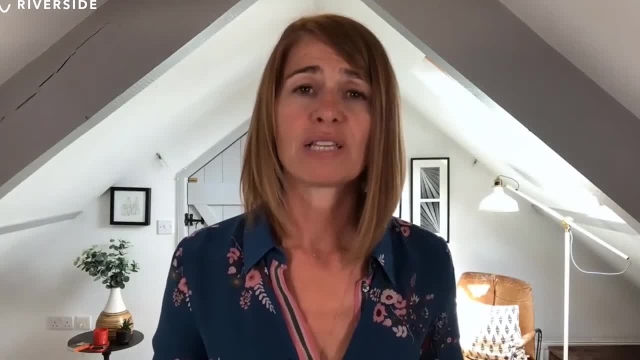 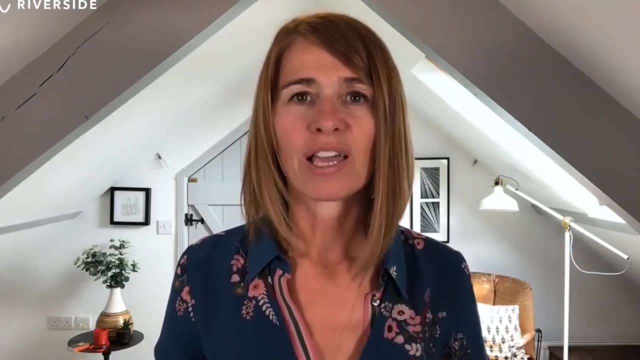 So credibility In the moment. So ethos, uh, lived in. ethos is really about: are you credible in life? So do you do this, the things that you say you're going to do? Are you a truthful person? Do you live by your morals? 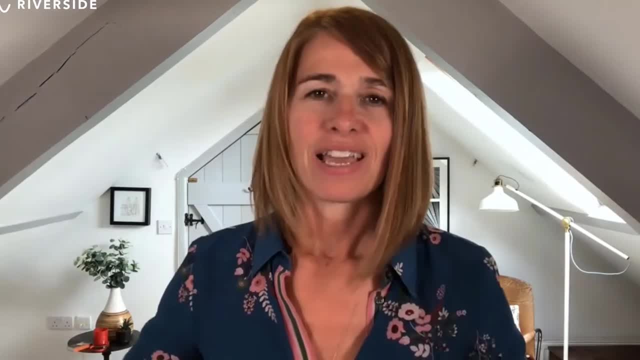 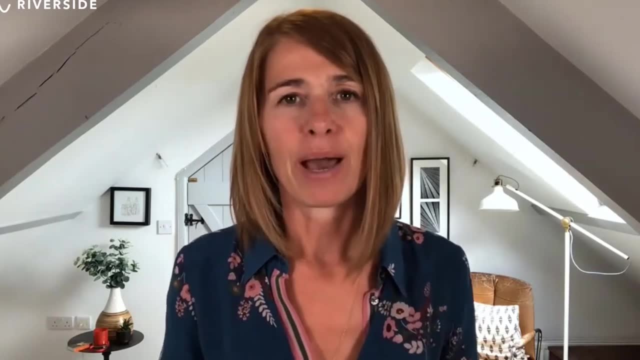 Do you walk your own talk. So that bit is really how you live your life And to some degree we still really rely on this. You know, look how upset we get about politicians who flout the rules, who do things that don't you know, say right. 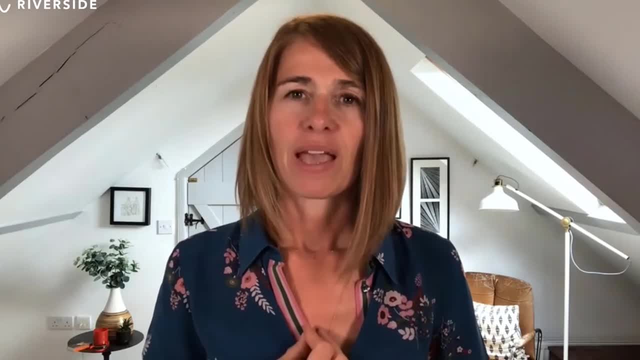 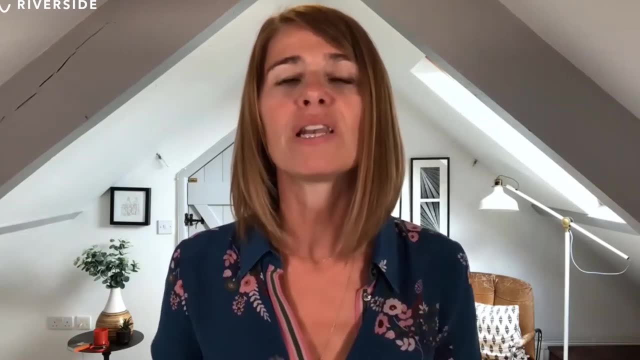 This applies to all of you, But I can do my own thing. How upset we get about that. They're basically breaking that ethos rule. They're breaking the credibility rule. They're not living by the rules or the instructions that they think everybody should live by. 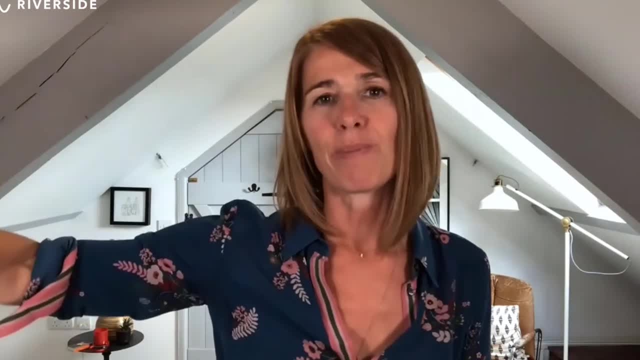 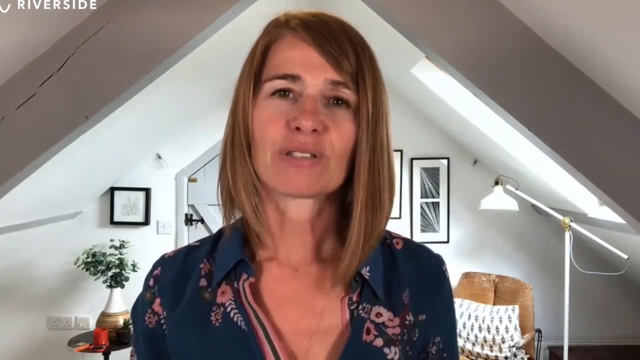 So that's a really important part And, again, this is where your back catalogue of work will come in, So if you've always done a good job, then that really is going to support your lived in ethos Now ethos in the moment. 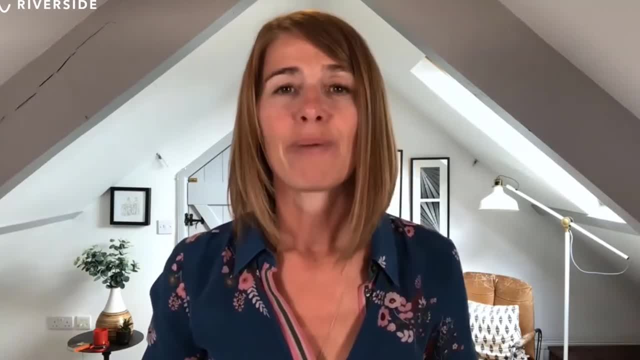 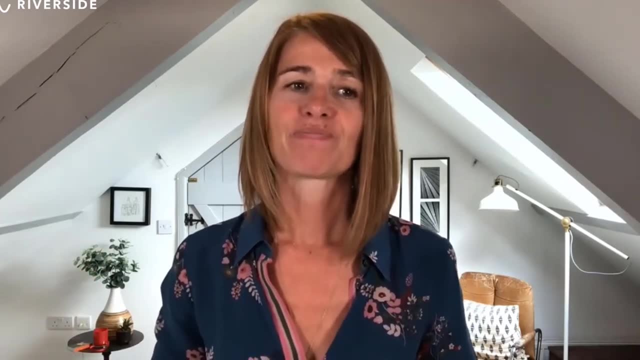 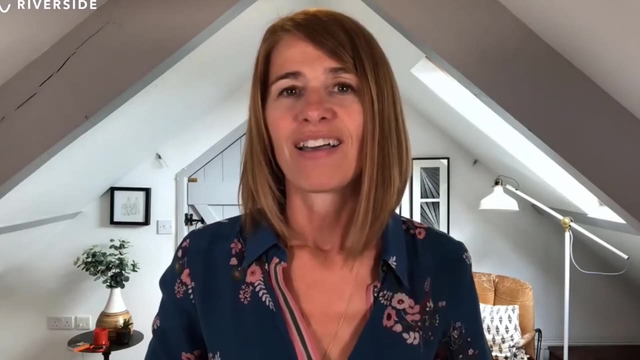 So credibility in the moment Is really about what you're thinking and what you're doing with your body, your breath and your voice in the moments of speaking. So body posture really, really important. Your audience will make a decision about how credible you are by how you sit, stand, walk, gesture, move. 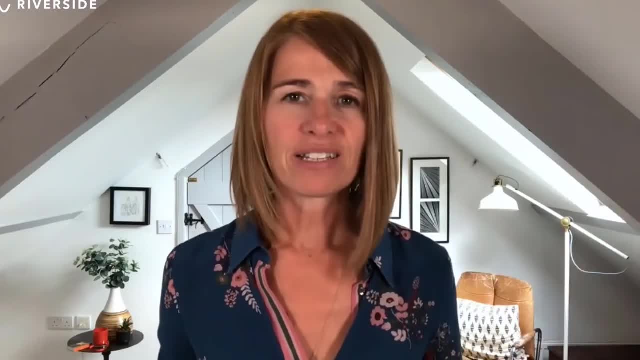 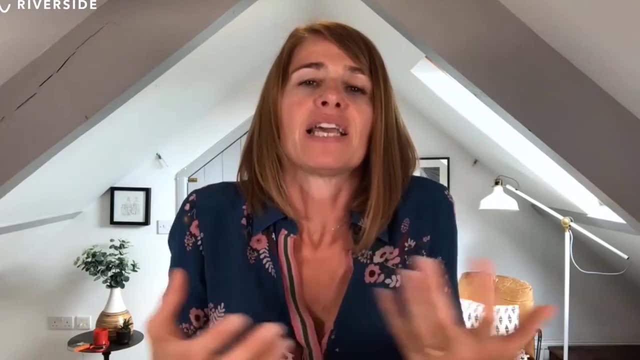 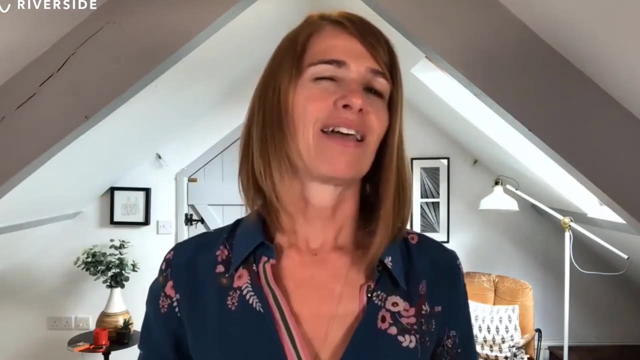 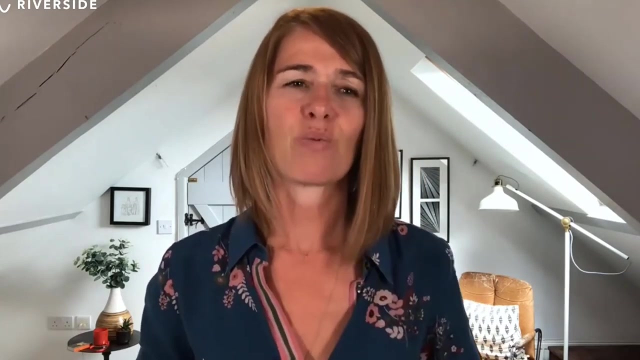 So we want your body posture to be open, relaxed, authentic, real in front of your audience. Yeah, if it's the opposite of that, If it's tense and tight And you're not really being authentic or you're being overly confident, your audience are going to pick up on that in a second and they're going to know that that's not quite true or real and they will recoil from it and not really understand why. 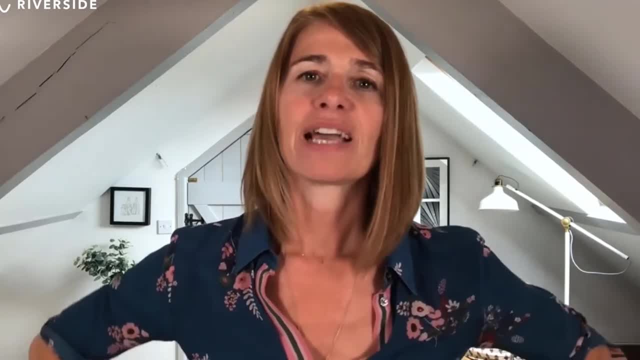 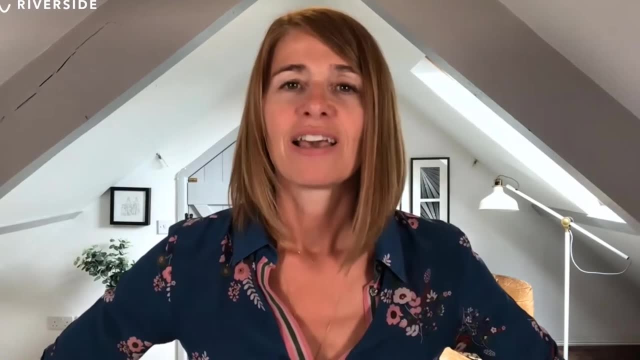 Now, the second thing is that your breathing needs to be really deep and relaxed. So when we get nervous, anxious and speaking at team meetings in public and doing pitches, you know when the stakes are a bit higher- Our breathing can get a bit up here, so it can move up into our chest. 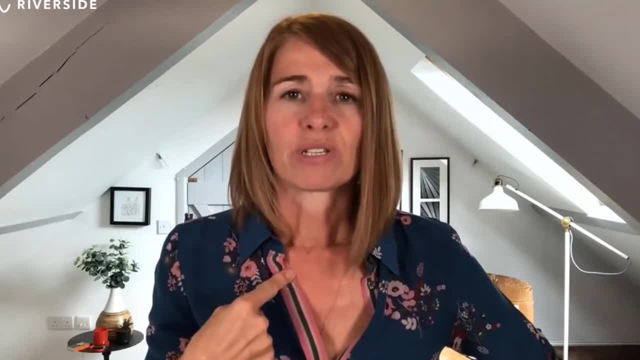 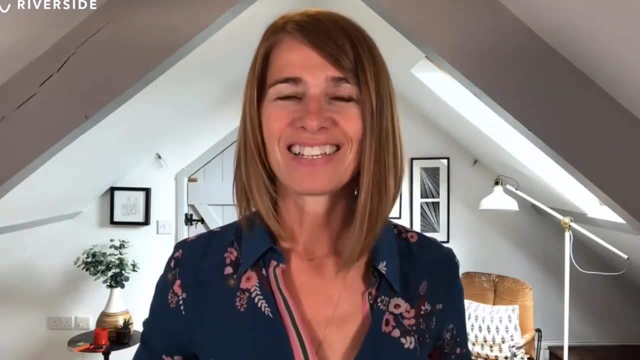 Now, the moment that we start doing that, we look nervous to our audience. Our audience starts to feel nervous on our behalf. So we really want to make sure that the breathing is low in the body centered. It helps us think more clearly, gets blood and oxygen to the brain, which we definitely need. 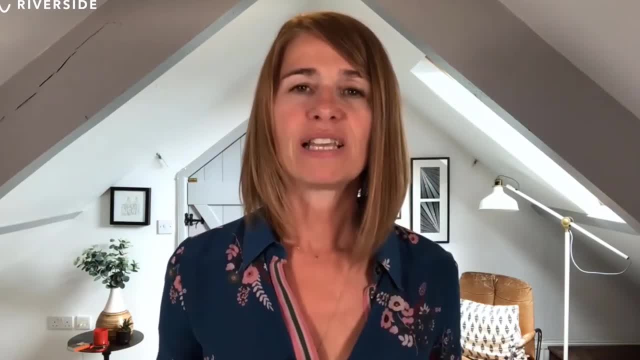 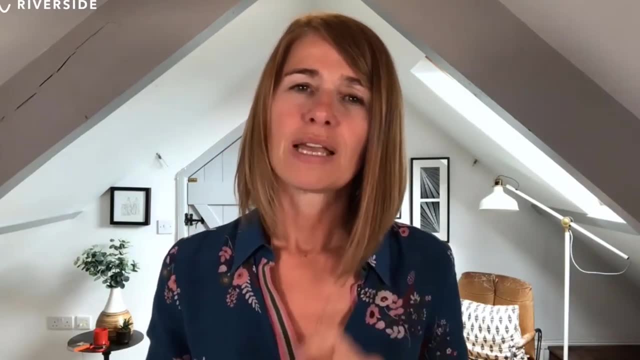 So, by standing well and breathing deeply, our audience go: oh, okay, I can trust this person, They're okay, They know what they're talking about. And then we start to move into things like gesture and tone of voice. So, as we've said in other videos, go watch. 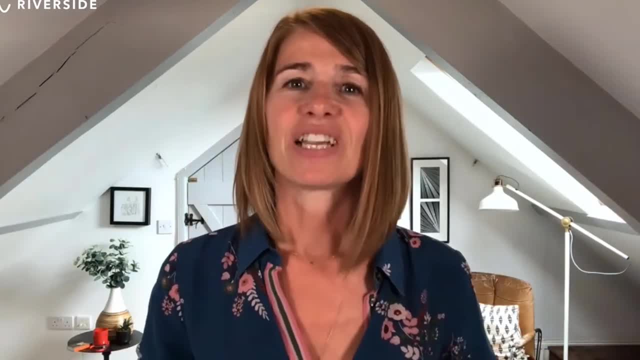 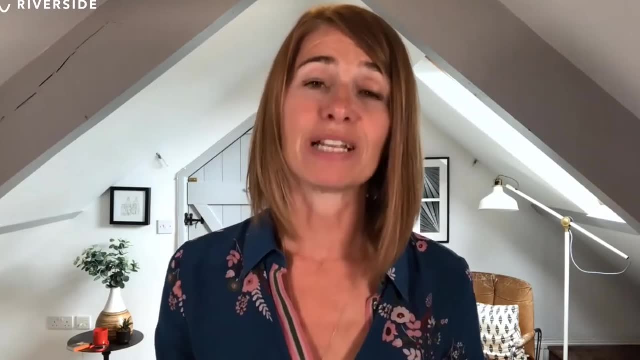 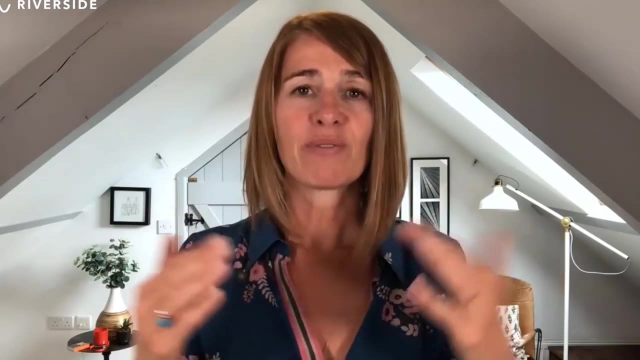 There's a great video on what to do with your hands when you're speaking. Gesture is absolutely vital to help with your personal credibility and the memorability and the actionability of your content And, equally, tone of voice is ever so important. So if I raise my voice and I disembodied my voice, it now sounds like it's coming out of my head. 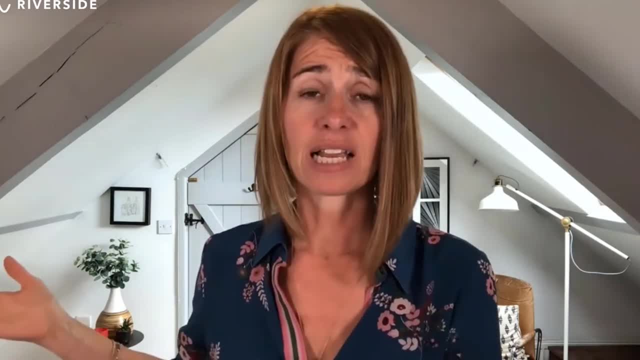 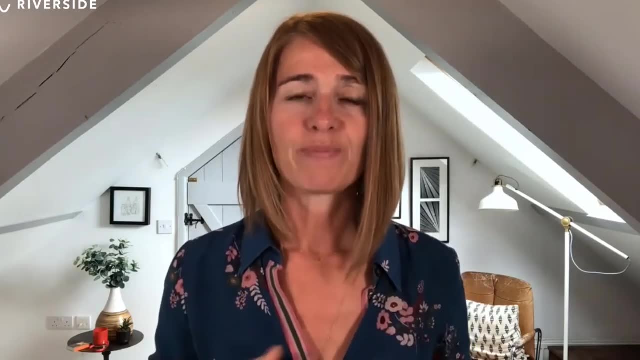 So I still know as much as I did A second ago. I just don't sound like I do now. So if I relax and let my voice drop back down into my body, so now it's in it what we would call an embodied voice. 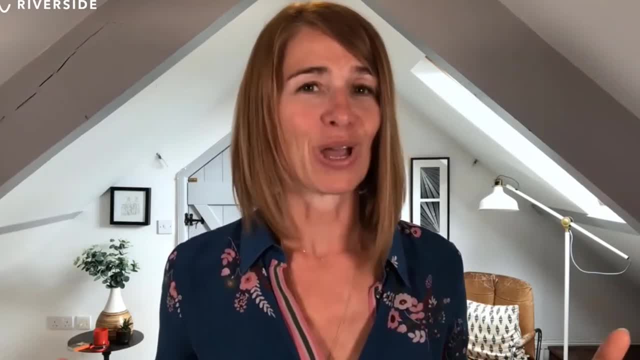 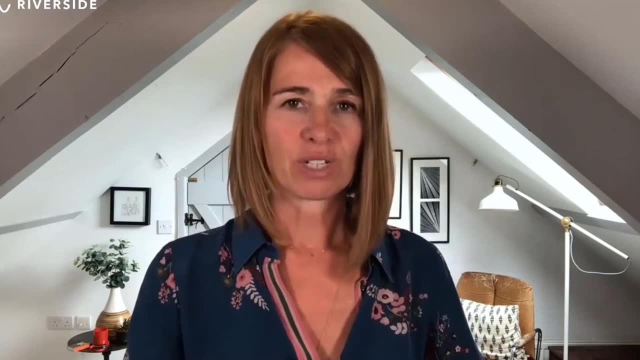 I suddenly sound like I really know what I'm talking about, or at least I hope I do So. I sound like I know what I'm talking about. My voice is coming out of my body. It's easier to hear, listen to and respond to without feeling a little bit stressed or uptight. 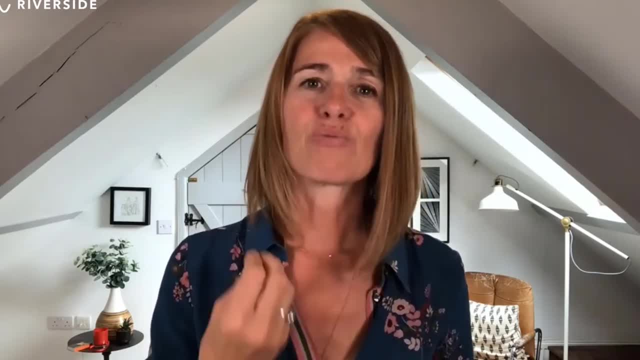 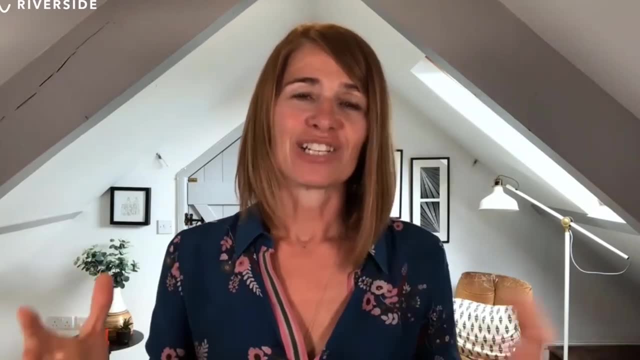 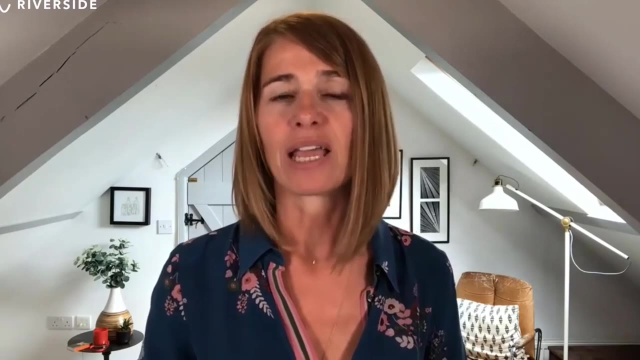 So we want to make sure that the vocal quality is really powerful, Really is Really impactful and genuinely your voice Okay. Now intonation is ever so important, So that's the sort of up and down-ness of your voice. So if I continue to do the rest of this video without any up and down-ness, you're going to get pretty bored within a sentence or two. 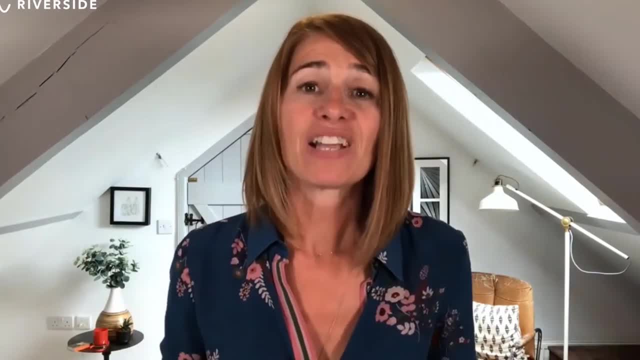 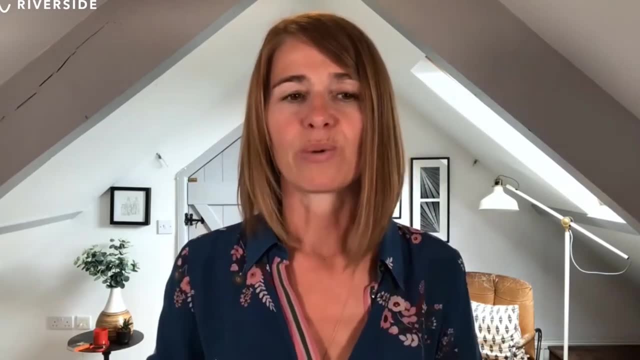 So we really need to feel the passion, the energy, the connection with what we're talking about, And if we don't feel that, we're going to get pretty bored pretty quickly And then finally pace and pause. So if you stand up on the stage and you rush and there's no pauses and we keep going really, really fast. 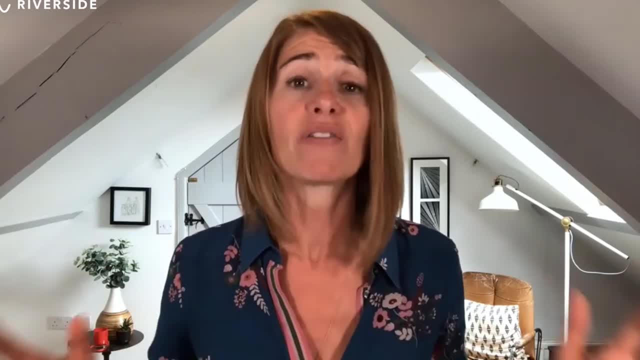 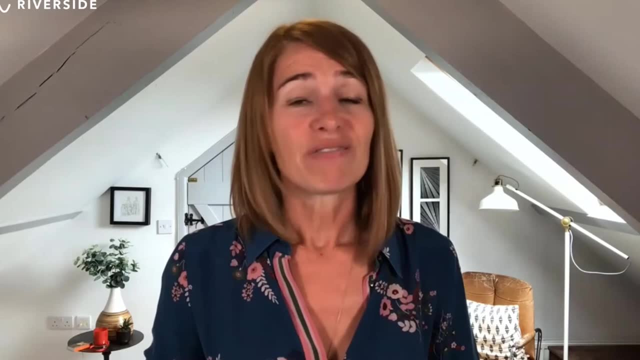 So my pace is way too fast and there's no pausing, And so it's really really hard for you now to get a grip on my content. It's really hard for me to get a sentence out fluently, So I don't look or sound credible or in control of my material when I'm speaking too fast and there's no pauses. 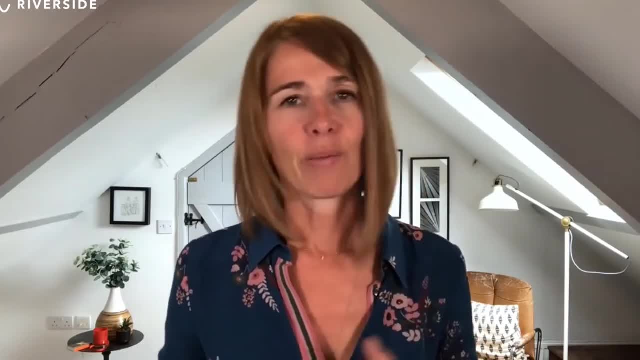 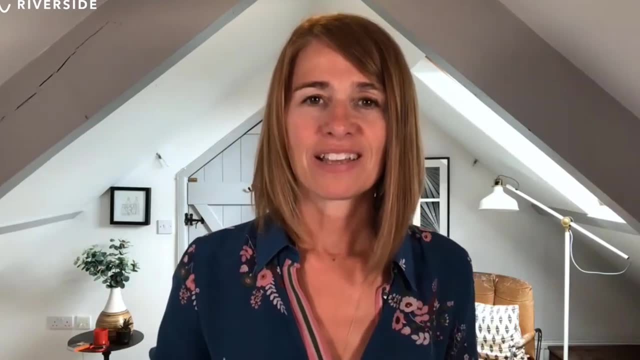 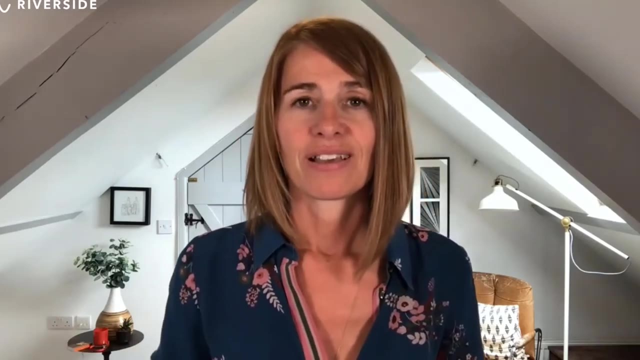 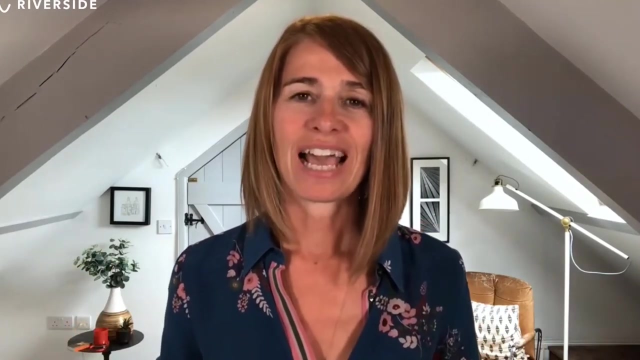 And if I don't pause I can't breathe. No blood, no oxygen, Thoughts get muddled. So all of those things together- How we stand, how we breathe, how we gesture, the tonality of our voice, the intonation of our voice, our pausing and our pacing- are all really important to how credible we sound as a speaker. 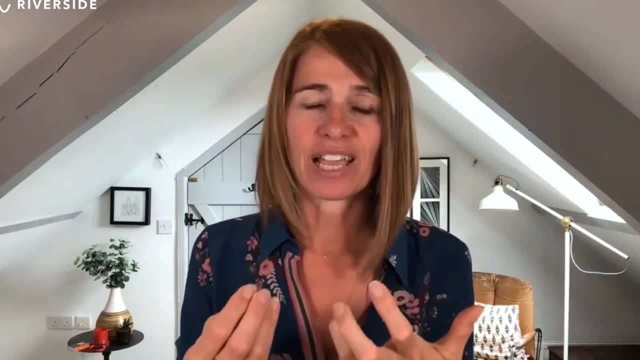 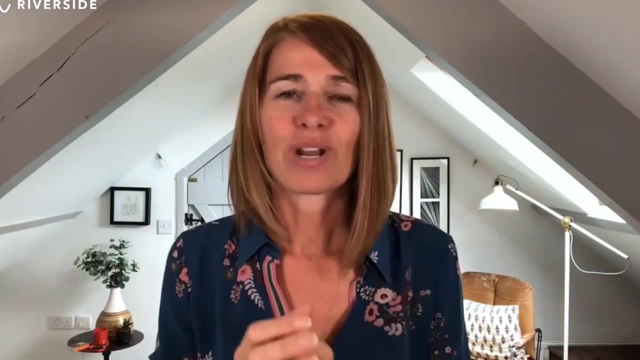 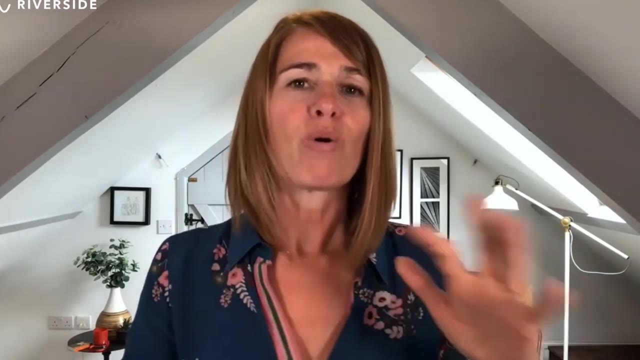 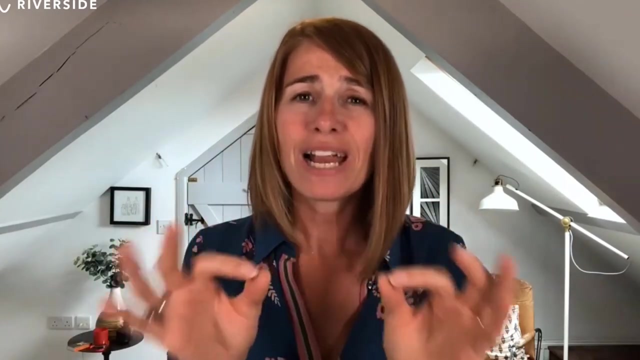 And when we can manipulate those things purposefully, intentionally, then we can create incredible presentations and pitches and stories and updates- in whatever ways you speak to your audiences- That are really, really impactful. But if we don't know what all those elements are and we don't know how to manipulate them and use them to our benefit to make it our messages, really understandable and memorable to our audience, 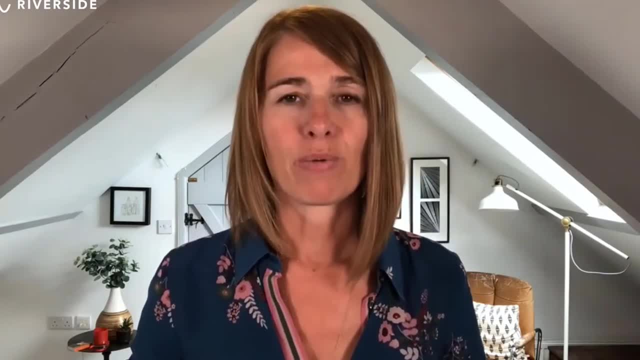 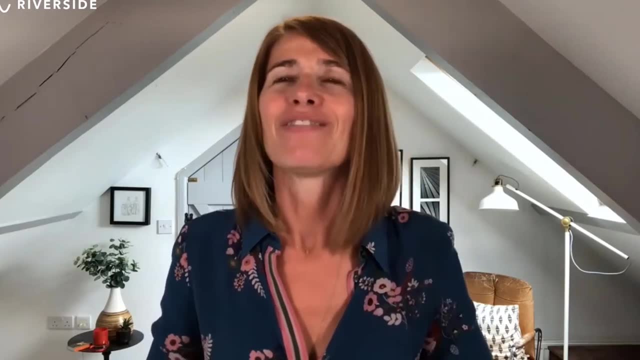 It's pretty unlikely that they're going to remember what we've said, action what we've said or perceive us as credible. Now, I love this work. I think it was an incredible thing that Aristotle did. I think it was a complete gift. 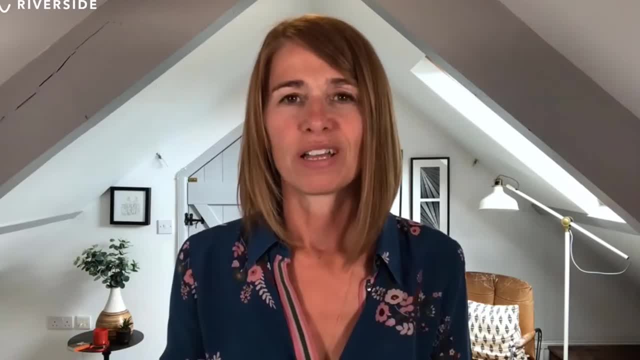 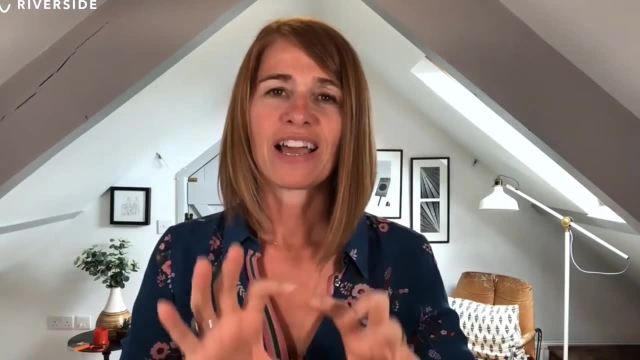 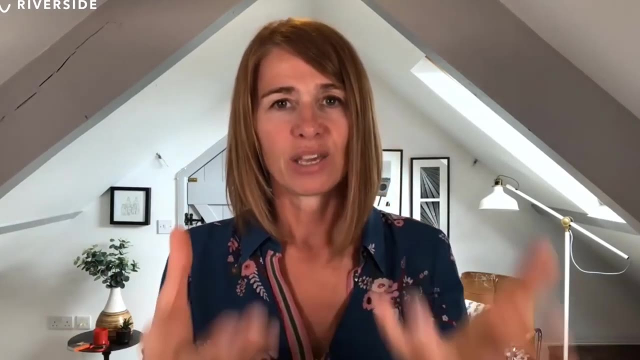 It was incredible And, like I said, I've never really found a model that emulates this simplicity and this effectiveness. So I took this model and I have created the speaker credibility assessment, Because for me, it's really important that you, as a speaker, know where you are. 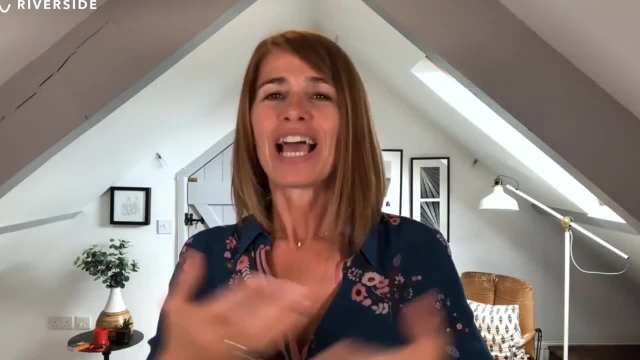 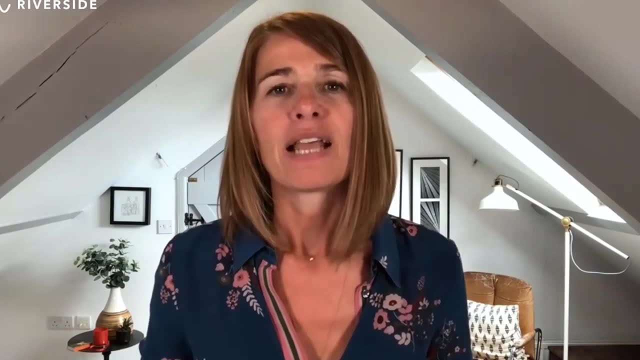 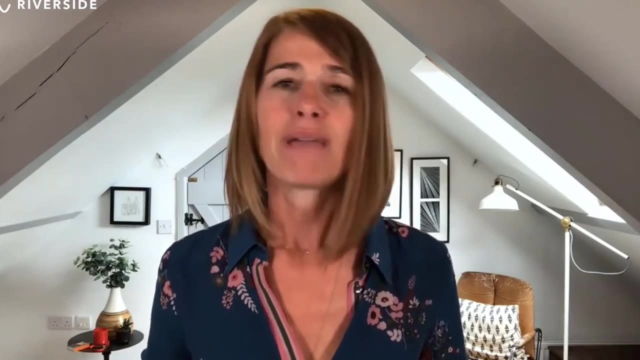 It's a bit like having a map You know. unless you've got a map, you don't know where you've been, You don't know where you're going. You really need to know where you are Now. One of the reasons that I created this speaker credibility assessment is because over the years, I've had many, many people come to me saying: oh, I'm a terrible speaker. 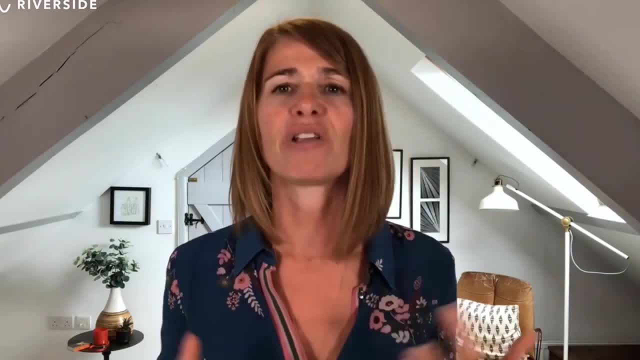 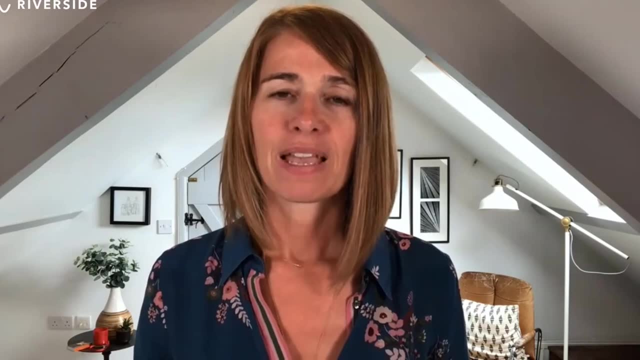 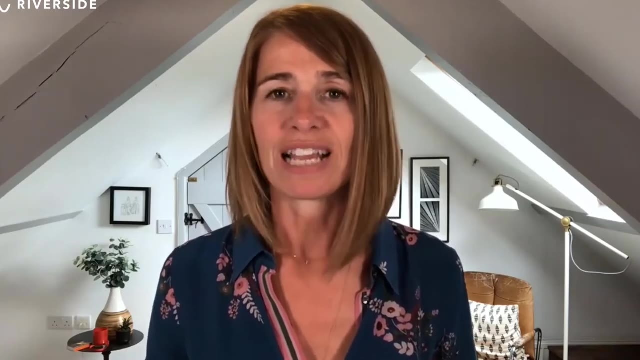 I'm awful at this and I hate presenting and I get so anxious and so nervous and everybody can see it And they tell me a laundry list of things that they're rubbish at when it comes to speaking And, in my experience, when I listen to them speak, there's usually an equally long laundry list of all the things that they're doing brilliantly. 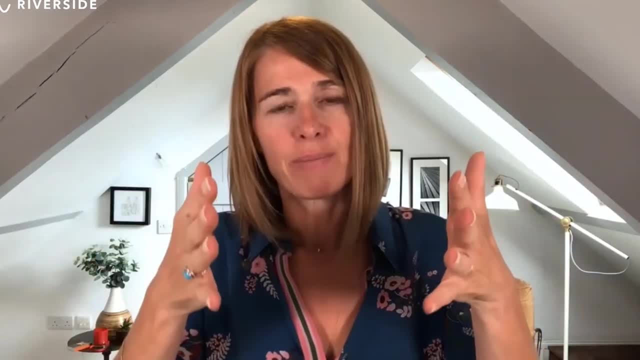 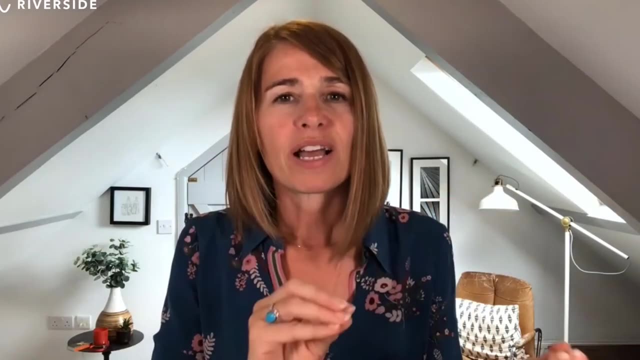 It's just they're stuck in that moment of not being able to see the good stuff. They can only see the bad stuff when they look at themselves. So one of the reasons I created this was to be able to tell people: look, you're already doing this brilliantly. 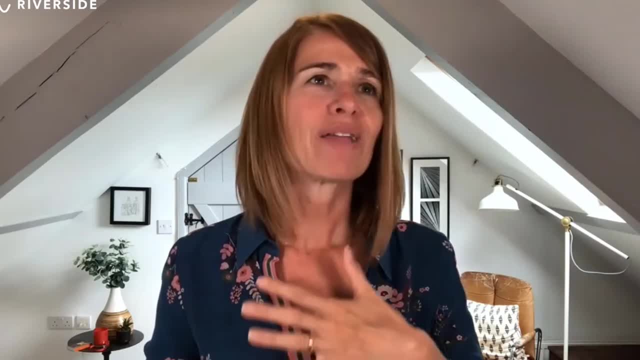 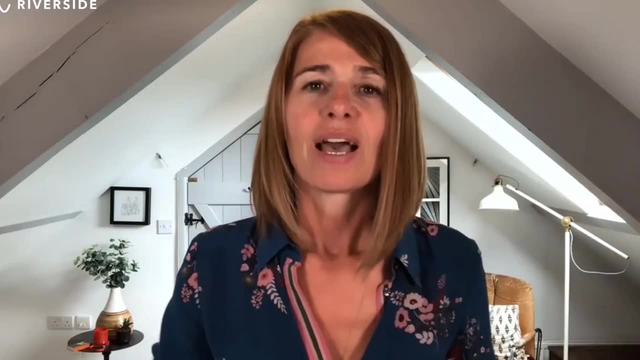 You've got a beautifully warm tone of voice. You have an amazing way of making eye contact. You tell gorgeous stories, So this is all really really good. We might want to work on these things over here, but these things are excellent. 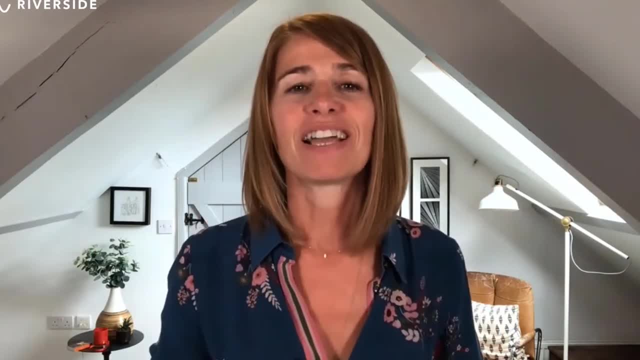 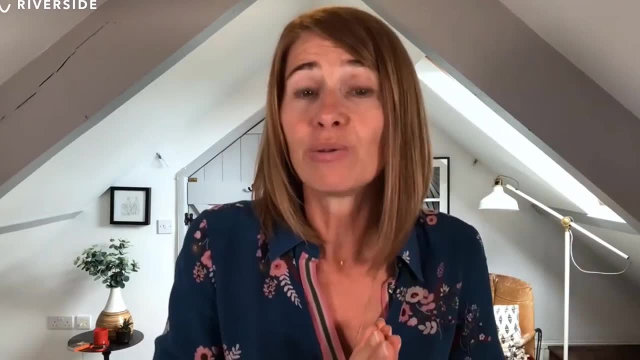 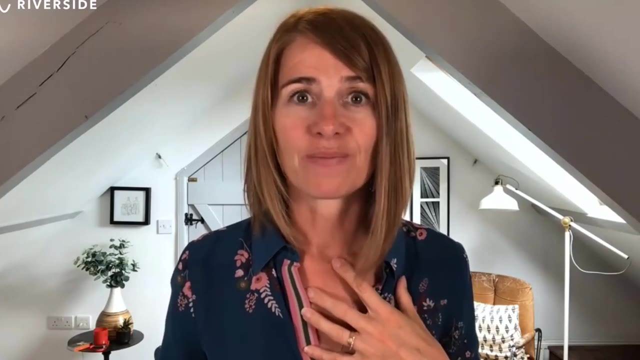 So I'm going to show you. So the speaker credibility is designed just to do that. It's designed to show you what you're already doing really, really well. And I promise you, even if you think you don't feel like you're a great speaker, there will be things that you're doing really well that your audience will appreciate. 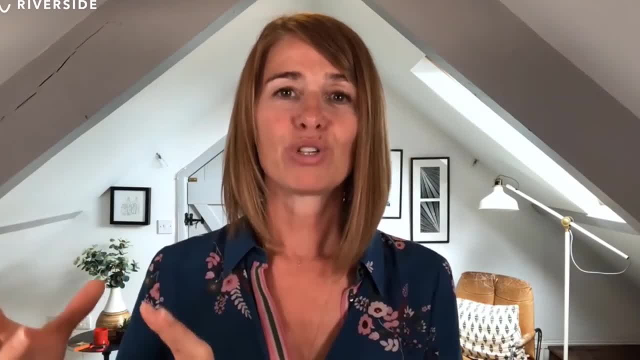 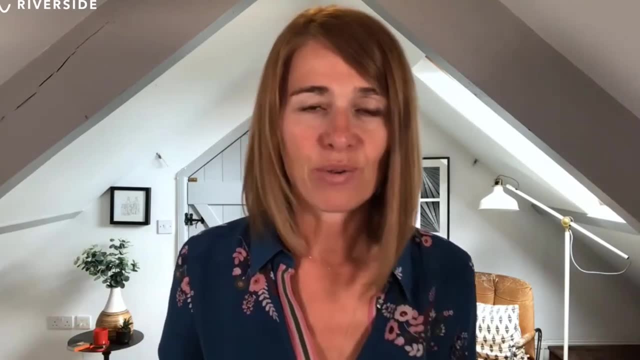 Then, on the other side of that, it's designed to help you show- to show you, rather, some things that you maybe want to reduce doing because they are detracting from your message or they're detracting from your credibility Or they're detracting from your impact. 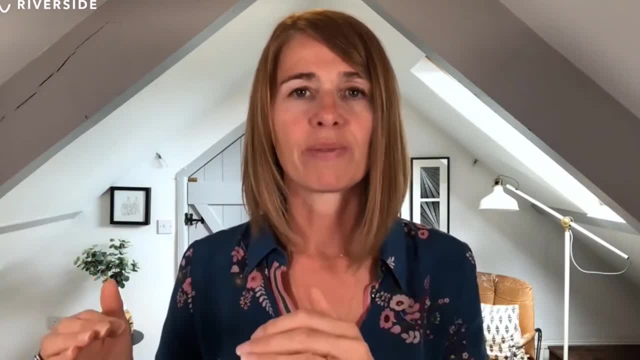 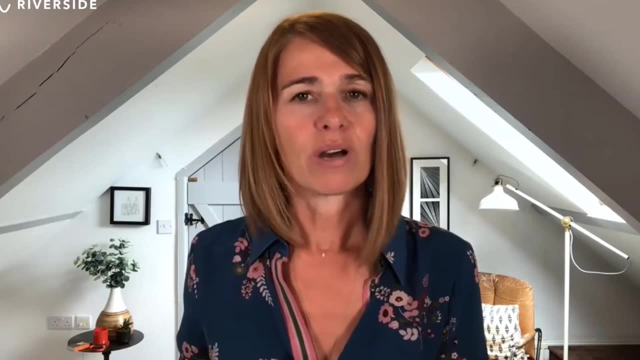 So we might want to just reduce them- not necessarily stop them, but reduce them- And then there will be one or two things that we definitely want to stop doing because they are genuinely undermining your credibility and they're making a big negative impact on what you're saying. 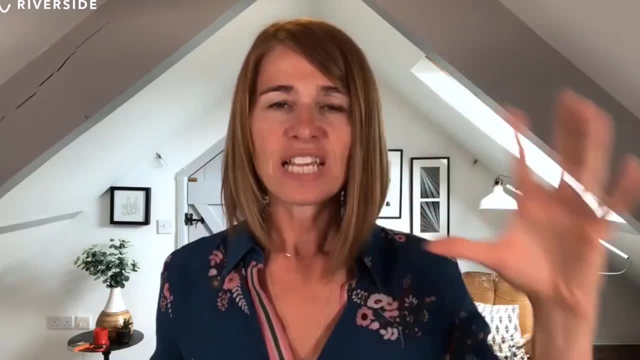 So that's the way we look at the voice. We look at it across 15 data points And we're looking at your body, posture and all the things that I've talked about today, And we're looking at your ability to create that connection. 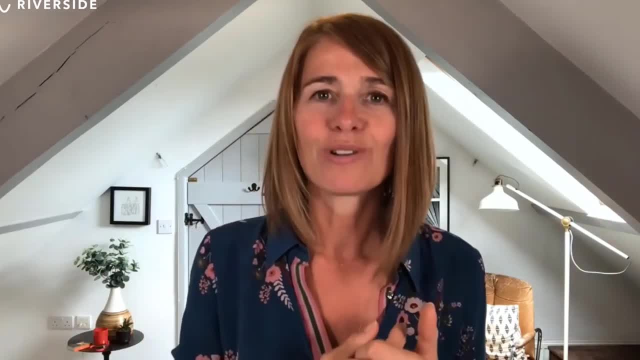 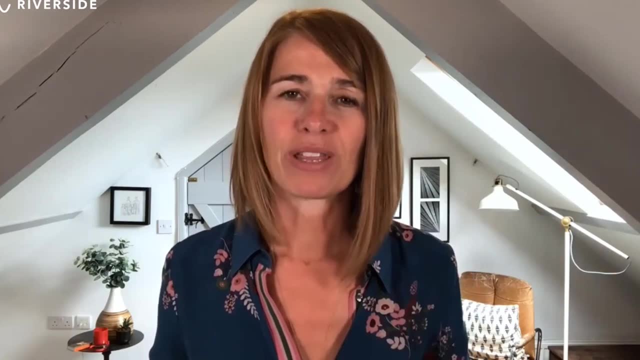 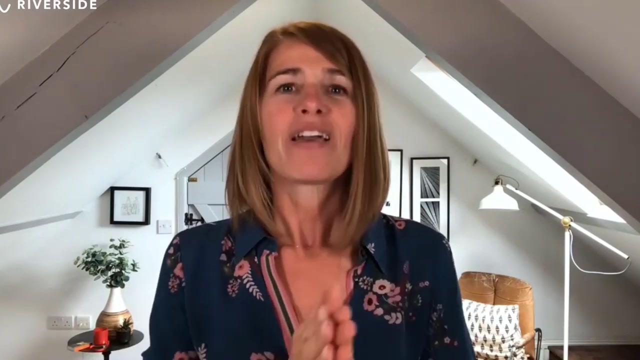 Create that connection with human beings, your ability to be logical and make a really clever, flowed argument, And we're looking at your credibility in terms of your body, your breath and your voice and what you're doing, And we create a report. So we create a video based on your essentially what you're going to. I'm jumping ahead of myself. 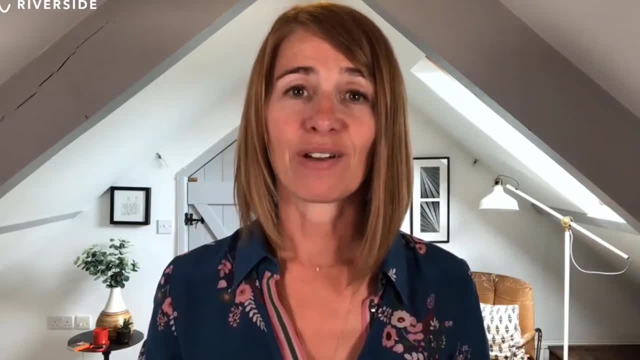 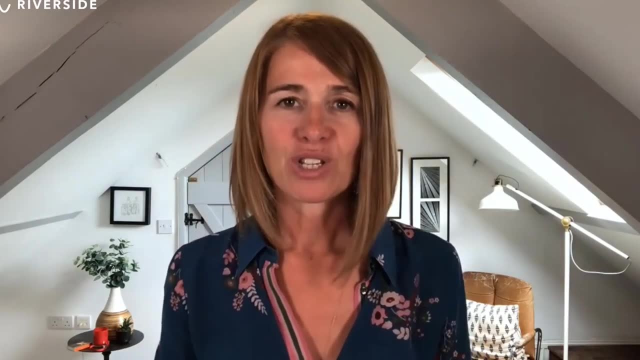 Essentially, what's going to happen is you send us a two minute video of you talking, and it can be you doing your networking pitch. You could be talking about an amazing vacation you went on, It doesn't really matter, But you send us a two minute video just on your phone, as long as we can see and hear you. well. 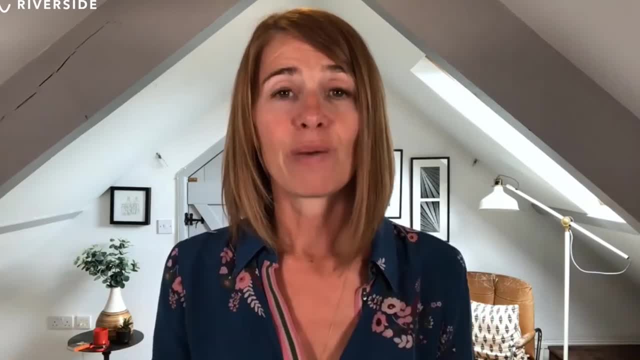 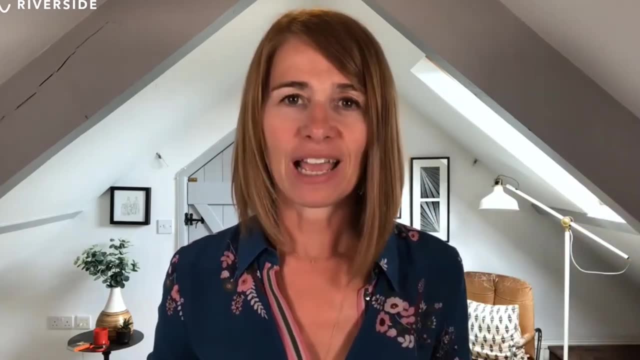 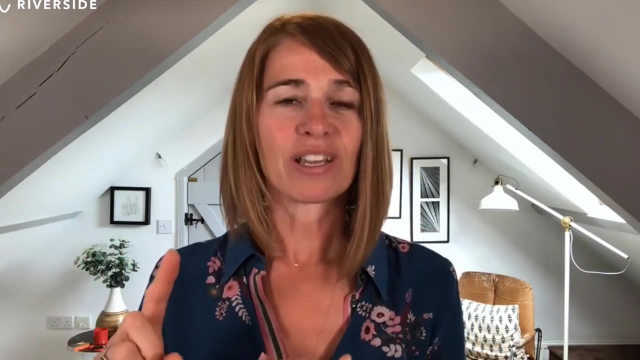 That's all that's necessary. Then we will send you a video back showing where you're doing a brilliant job- So all the things that you are already doing brilliantly, based on emotional connection, logic and flow and your credibility- And then we will look at the things that you could reduce doing or stop doing to increase your impact. 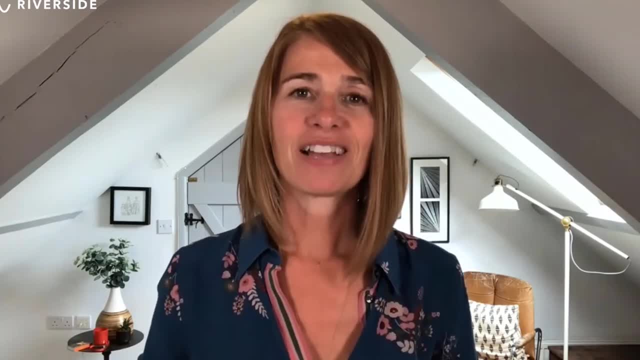 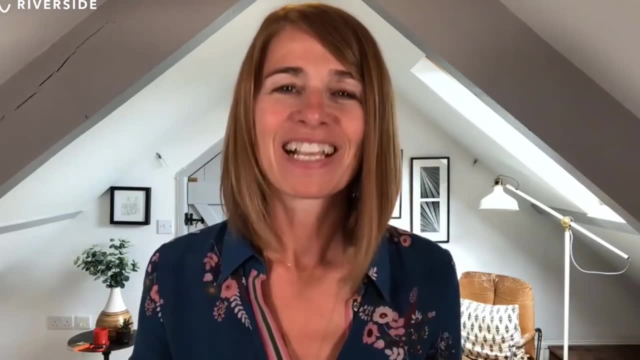 If you're interested in getting a personal assessment, A personal assessment, a personal speaker credibility assessment- We would love to help you out. As you can see, I love talking about this, So there is a link below. If you'd like to take our speaker credibility assessment, please click the link. 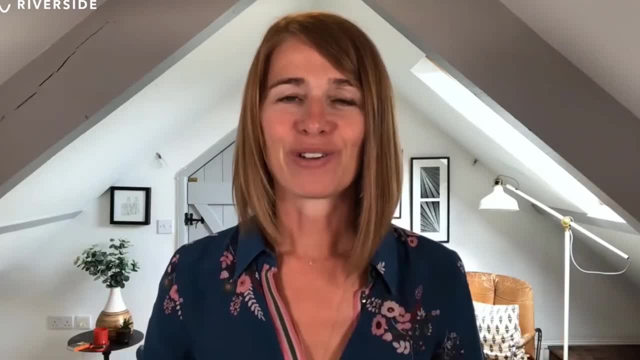 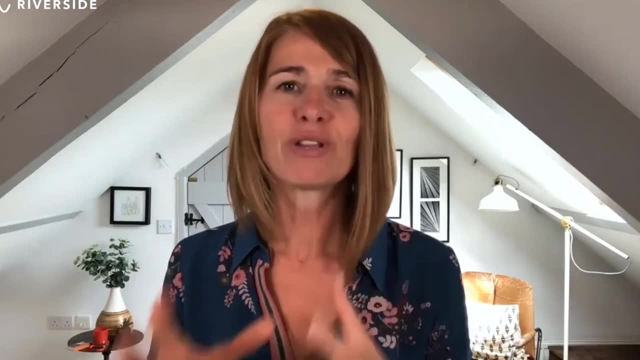 Follow the instructions and sit back and wait for your feedback. If not, I hope you found today really really helpful. So the next time you're preparing a presentation, I really want you to think about emotional connection, logic and flow And how you're going to tell your audience. 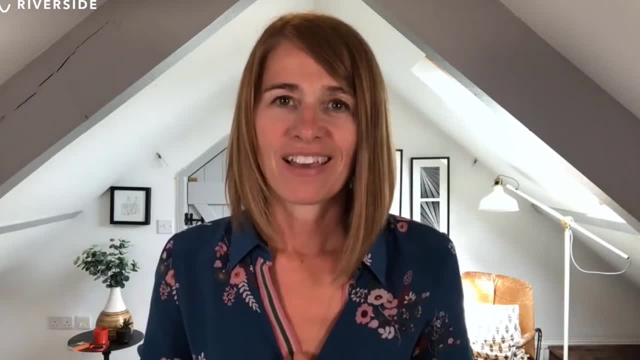 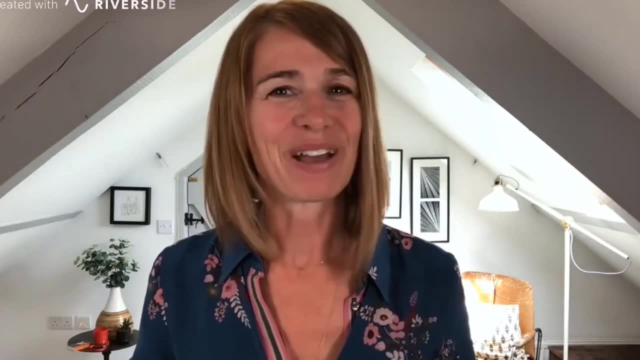 The story. How are you going to be, How are you going to support the message that you're giving? Take care and we will speak very soon. Bye for now.